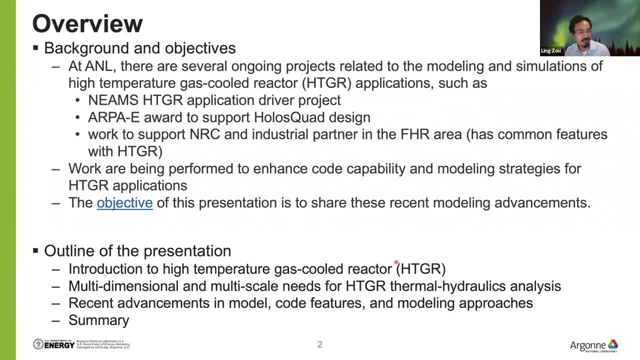 So before stepping into the presentation probably want to give a little bit of background and then the objectives of this presentation. So at Argonne National Lab So there are several ongoing projects that are related to the model and the simulation of the high temperature gas cooled reactor applications. 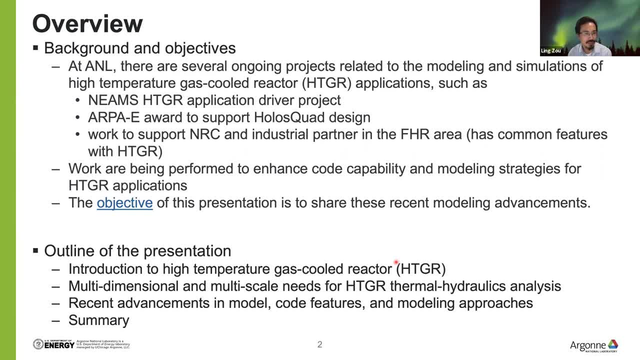 So we have NIEMS HTGR application driver project, which is a main focus on the system analysis and also CFD validation And also to develop the code and then apply the codes. I mean NIEMS code for HTGR applications. And we also have another project, APA-E awards, that are to support the Hollis quarter design. 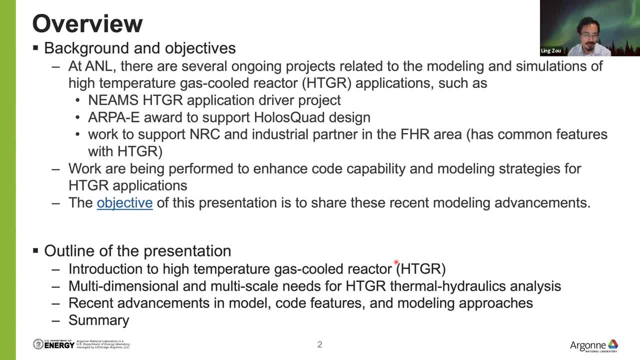 The Hollis quarter design is also HTGR design. It's kind of innovative. It's a horizontal design but it is a prismatic design. So the purpose is to make the reactor small. They can fit into an iso-condenser. The container can be easily transported. 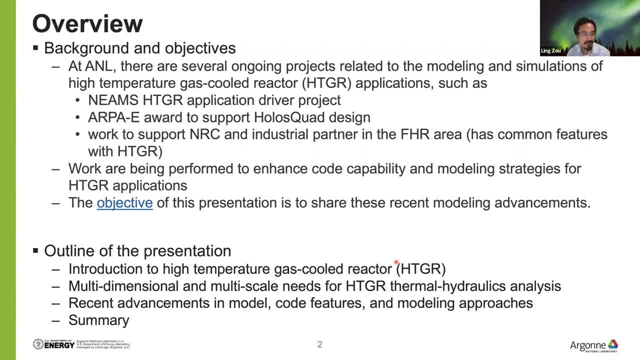 And we also have a work to support the NRC and our industrial partners in the PBFHR area, Although, of course, PBFHR is not like the HTGR, but they do have a lot of like a common features which with HTGR. 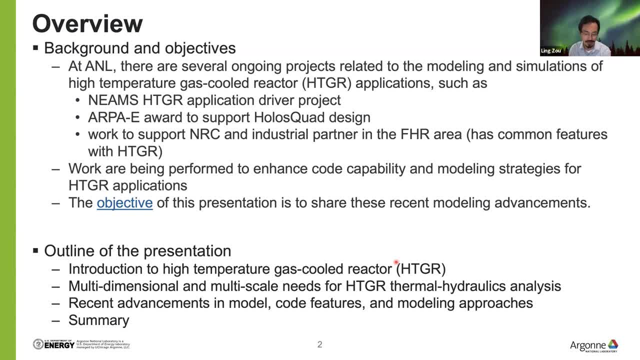 So that's why some of the work is also included in this talk. So at Argonne we are working to develop, to develop the code and also to improve our code capability and also how to model the HTGRs, And so the objective here is really to share this recent advancement with the community. 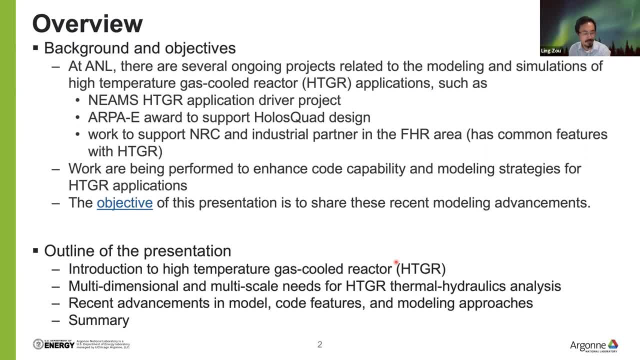 Like: what's the new code feature we have, how we have improved our way to model the HTGR, things like that. So with this, for the following of this, this presentation, I will briefly talk about the HTGR. I suppose you are all familiar with HTGR design, but maybe I can still share some very brief introduction. 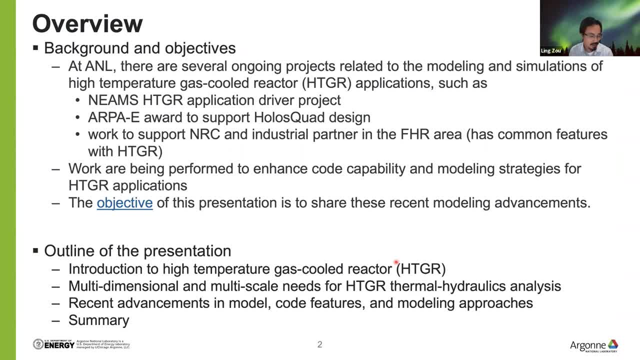 And then we will talk about why we need, why we need this multi-dimensional and multi-scale simulation capability for HTGR designs, And then, following that, we will then talk about the recent advancement in the model, the code features and the model approaches. 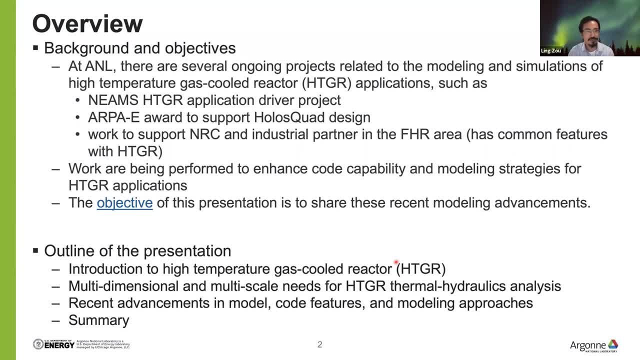 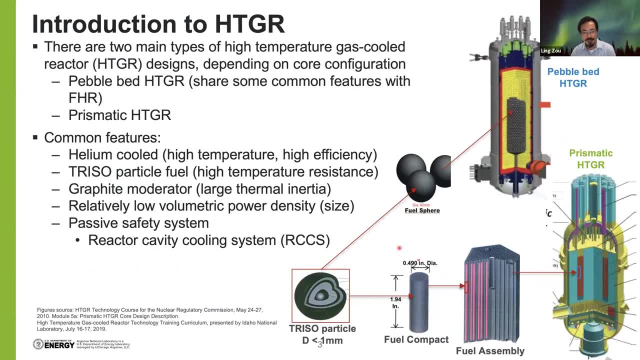 With that we will have a short summary. So introduction to the HTGR. I suppose everybody should be quite familiar with HTGR. If not, I can go do a quick introduction which is on the slides. So basically there are two types of, two main types of HTGR design. 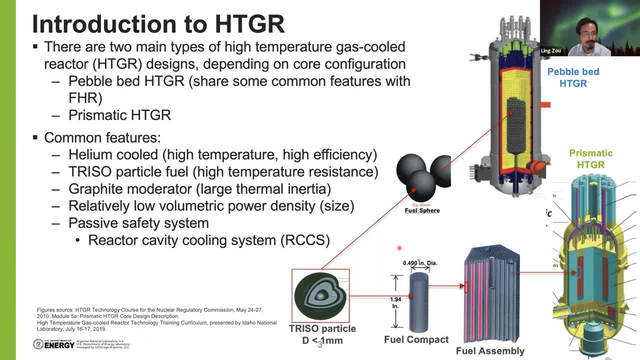 One is the so-called the paper bed and then the other one is the prismatic design. They should actually share a lot of common features If you look at the the, the trisor particle here. So they basically both of this type of reactors. they build upon this fuel technology and so-called the trisor particle. 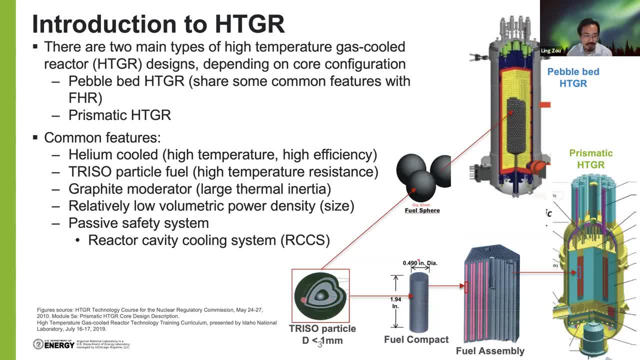 They are very tiny, small like particles with multiple layers with this fuel kernel inside. I think the the trisor particle is small And then one millimeter in diameter For the paper bed reactors. you pack this small trisor particles and then put them into this fuel pebbles. 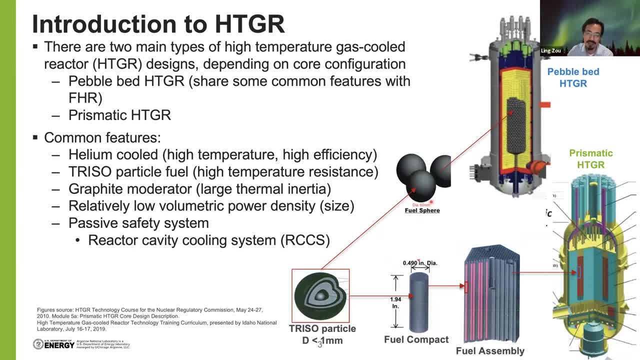 And then the pebbles is about like 60 millimeter in diameter And then you pack all this fuel pebbles into this so-called the paper bed, And then- this is why this HTGR is called the paper bed- HTGR On the prismatic. 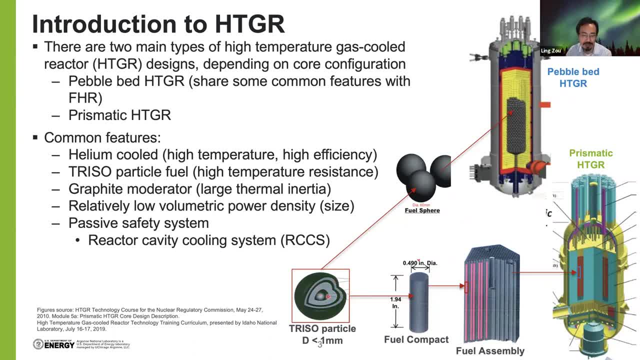 technical route. you have this, the same trisor particle, but instead of putting them in the pebbles you put them into so-called fuel pellets of your compact. So basically, compact the trisor particles with a graphite matrix And then you put this kind of like a pellet type of thing into this fuel assembly. 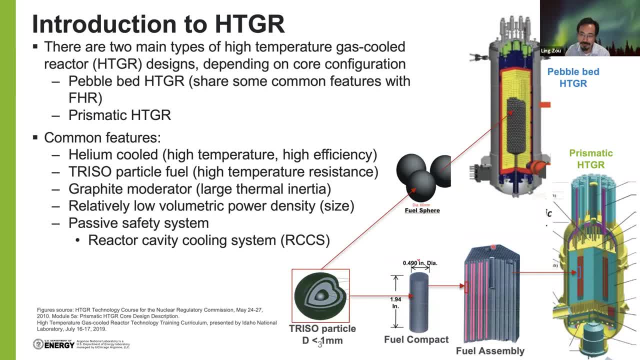 They are big hexagonal fuel assembly And then eventually you, you stack this fuel assembly into this core. So this is the so-called the prismatic HTGR. So they both of them rely on the trisor particle. the trisor particle. 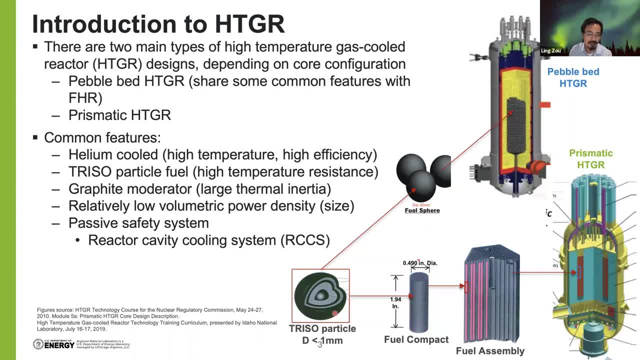 They they have very high temperature resistance, So so they so you can use them for this like a high temperature gas cooling reactor application and then use the helium as the coolant So the temperature can be very high. So, as we know, if you your coolant temperature goes high, you go higher efficiency. 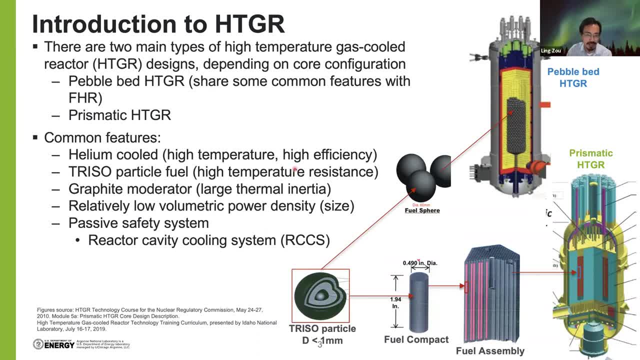 So, for example, in the light water reactor, we are talking about some efficiency in the 35 range, And for the helium core, the HTGR, the efficiency can go as high as I mean it can go at a minimum like 40%. 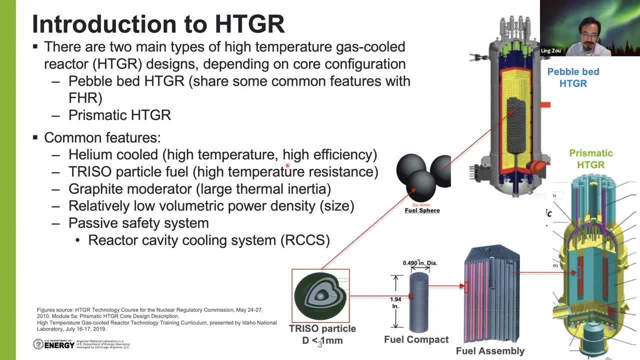 If you use like a Brayton cycle, your efficiency can go even higher, like 45%, And it's also used like graphite as moderator. So if you look at here, this yellow part is the moderator And then this, this green-ish color, is the graphite moderator. 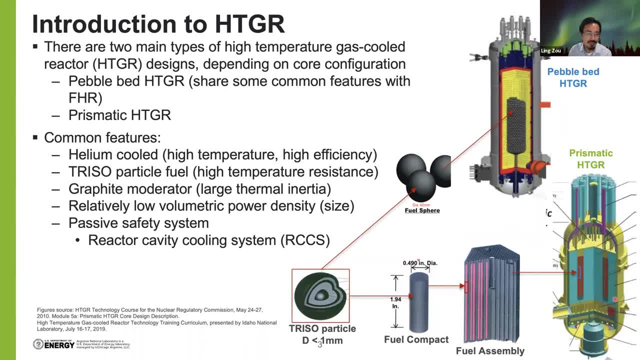 So they are of very large volume, which means they provide a very large thermal inertia, which is good in in in safety scenario, because larger thermal inertia will help you to smooth out your fuel temperature, the peaking temperature And both reactor type. they rely on the so-called the passive safety system. 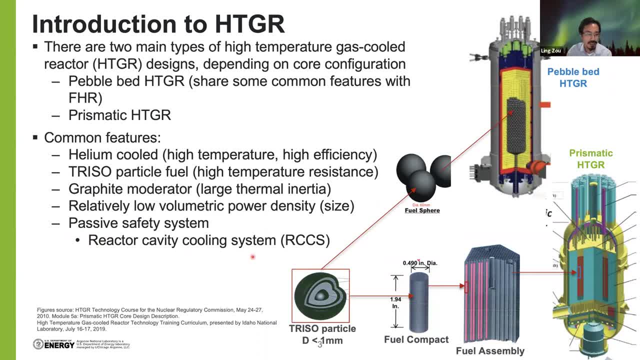 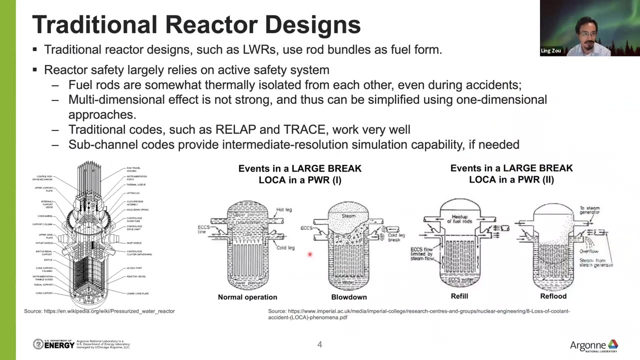 which is the reactor cavity cooling system. I will talk more details about the RCCS, which is a very critical difference between this advanced reactor and the traditional reactors. So before we go to the advanced reactor, we probably want to have a very brief look back at the traditional reactor designs. 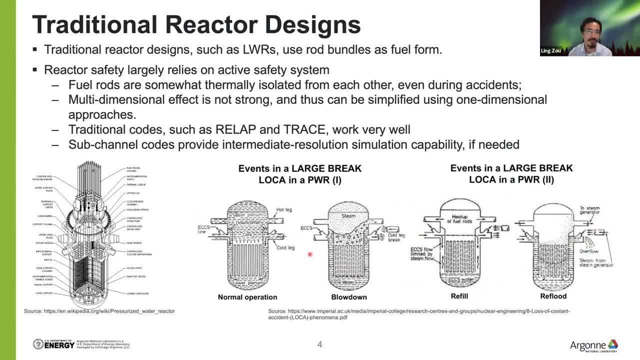 such as the AWR or light water reactor designs. So they use different fuels, They use different fuel forms, using fuel fuel rod bundles different than the pebble bed and also the prism, the prismatic block. So in this kind of core configuration, 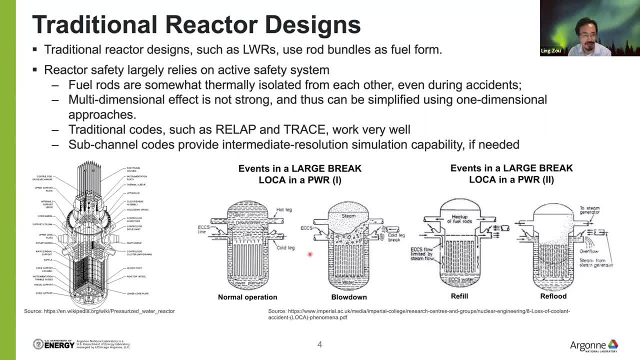 the fuel rods. they are somewhat similarly isolated from each other. So basically, similarly, they do not talk to each other, Even during a very complex accident such as the Lokon. So basically you are, you are losing your, your flow at the one of the bigger leak. 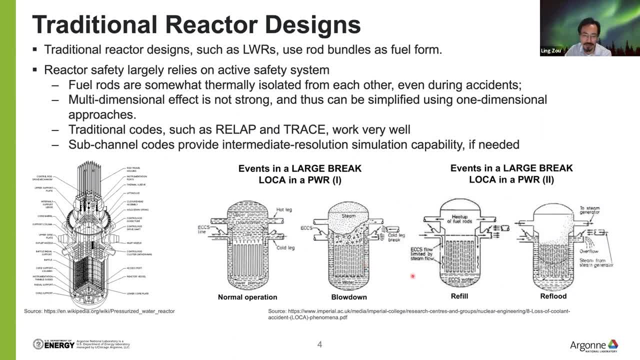 And then you, which is called the blowdown phase, And then you start to using your ECCS to refuel your reactor And then eventually, because it's very hot, and then it's like a single phase steam and then eventually you can reflood your core with a two phase flow. 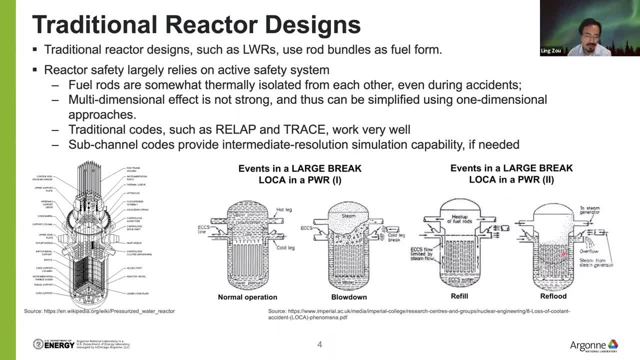 and then eventually the single phase flow. So you can see, this is probably the most complex accidents in the AWR, or in the PWR, let's say. But still, you see, the phenomena is actually still quite one-dimensional And the multi-dimensional effect is not so strong. 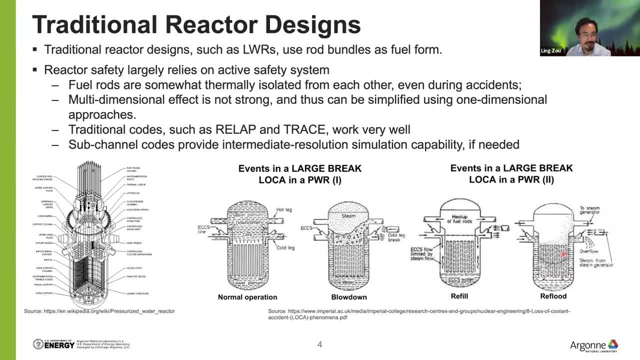 Of course they do exist, but they are not so strong, And then you can use some simplified model to model them, such as like a one-dimensional approach. So in this sense, the traditional codes like the relab 5 and the trace. they work pretty well. 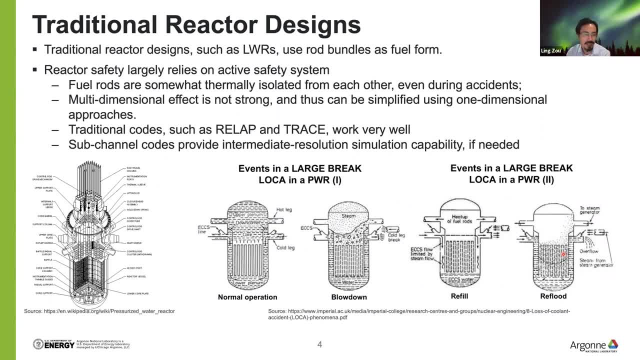 And if, in some cases, if you want to have them- higher resolution in the core but not going to the CFD, for example, you want to know where your hot pin is and then you want to have a better resolution to cover to your 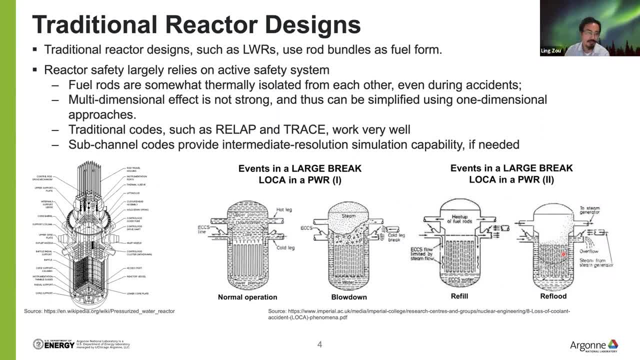 say react physics code to get a better picture of your reactor core, say to design your core, then you can go to the sub-channel code to provide this intermediate resolution simulation capability if it's needed. But if you look at the HTGR, 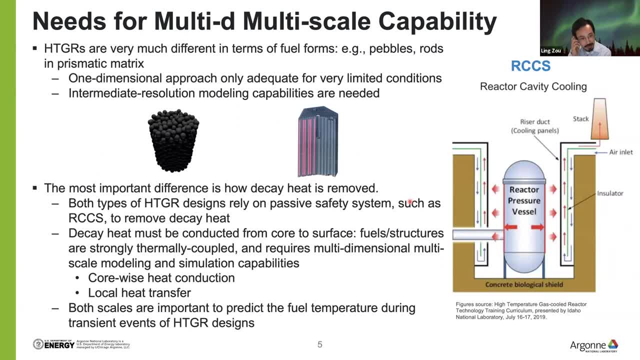 they're actually quite, quite different. I think we talked about the core configuration. So in the paper bed reactor we have this paper bed. In the prismatic design we have this, many, many in this kind of prismatic blocks. So in this case, 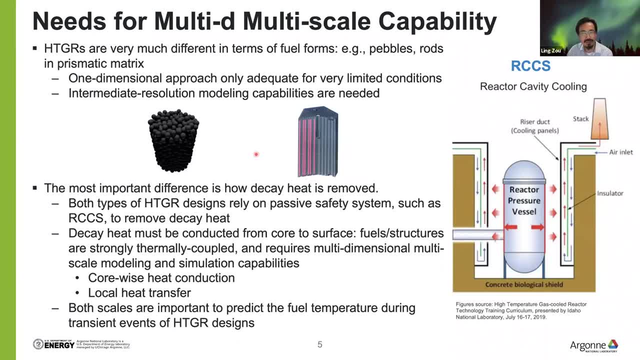 the one-dimensional approach. they are only adequate only for very limited conditions. First, if you look at the paper bed core, you can say: well, if the majority of the flow is going up or are going down, then it's probably okay to use some one-dimensional flow. 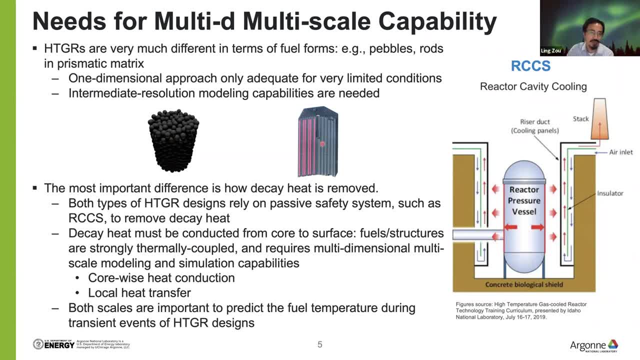 In this one. in the normal operating conditions it's probably okay. you have the, you know the flow in the one-dimensional, But we do not really have- I mean using system analysis code. we do not have a good intermediate resolution modeling capability. 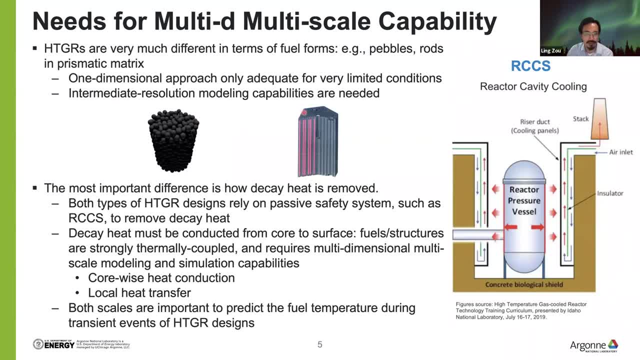 For example, if we really care about the, for example, the temperature distribution in this block, normally your system code cannot do not have such like a resolution. Another mostly important difference is how the decay heat is removed. So we just in the previous slides, 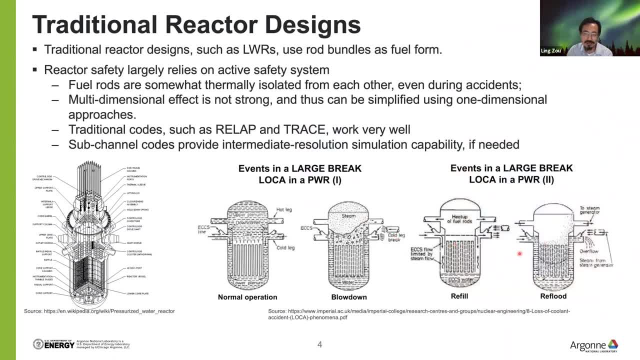 we mentioned that in this case, even in a very complex exit, then the flow is still pretty much like a one-dimensional. and then the heat removal mechanism is still the heat- I mean fuel- rod to the coolant Through the convection. 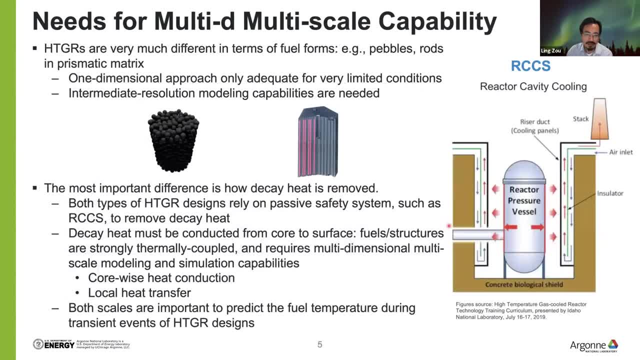 either single phase or two phase. But in the HTGR the decay heat removal mechanism completely changes. So basically it's from the center of the core and then go to the surface and then eventually go to the, the RCCS cooling panels. 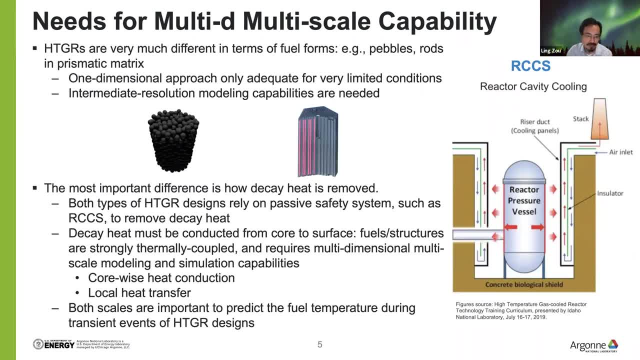 So there's two scales and the two types of heat heat transfer mechanism here. One is the heat core-wise heat conduction, Which dictates how your heat is moved from this core center to the surface. Another one is the local heat transfer. 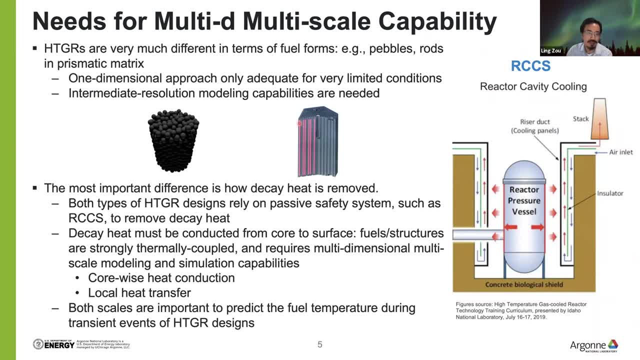 For example, if here we can see the localized heat generation and then the localized heat transfer dictates how your fuel picking temperature would behave. So both both scales are important to predict the fuel temperature during the transient. So that's why we need the 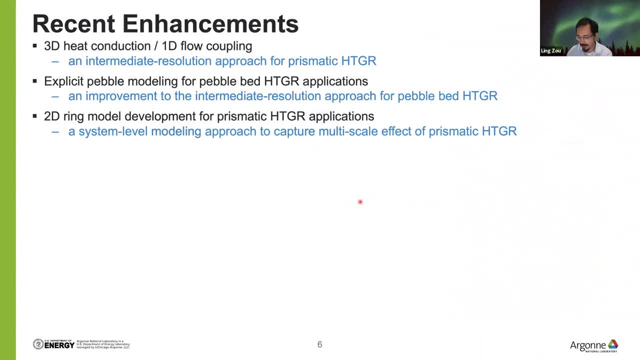 this multi-dimensional and multi-scale capabilities. So today the topic I'm going to talk about the three recent enhancements And then one is the so-called 3D-1D flow coupling. So it provides some kind of like intermediate resolution approach for the prismatic HTGR. 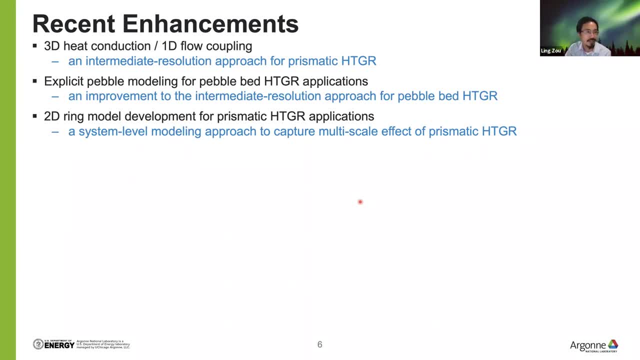 And then I'll talk about the explicit pebble modeling in the approach media approach, which is an improvement to the intermediate resolution approach. The last topic will be the so-called 2D remodel development for the prismatic HTGR applications. So this is like a system. 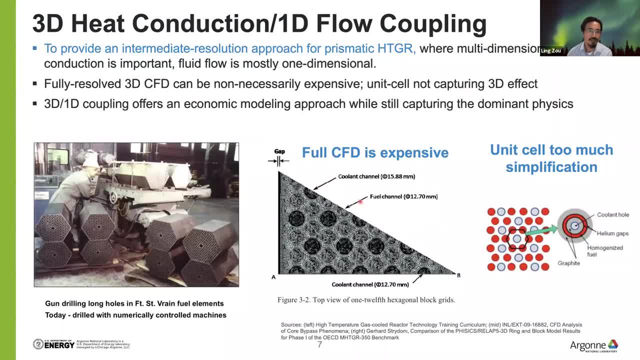 a real system level modeling approach. So the first one is the 3D heat conduction and the 1D flow coupling. So, as I just mentioned, it's really the main purpose is to provide an intermediate resolution approach for the prismatic HTGR. 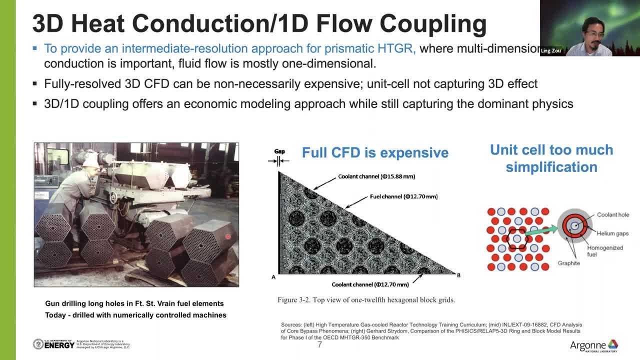 So if we look at the fuel assembly here, so you can see it's quite a big blocks, And then you see a lot of like holes drilled into this block. Some of them- like half of them they are for fuel pellet and half of them for coolant channels. 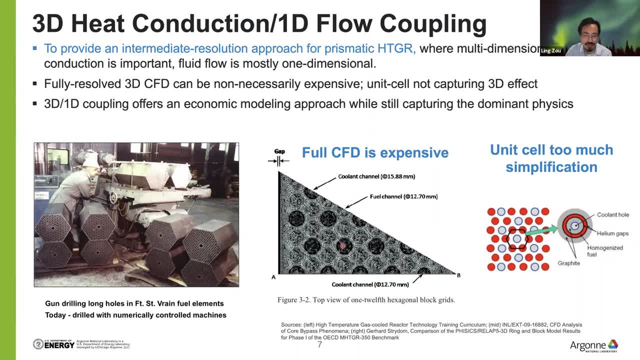 You can see probably clear here. So this is coolant channel and then this is the fuel pellet. So in this kind of scenario, especially during the normal operating conditions, there's actually not much of like an interesting phenomenon happening in this coolant channels. They are simply 1D flow. 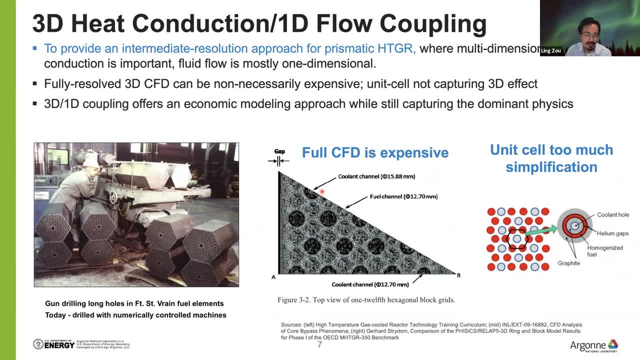 But if we want to go to the full 3D CFD then you have to resolve them using a lot of mesh, because we know if we want to capture the heat transfer in this coolant channel then we have to use a lot of mesh to resolve them. 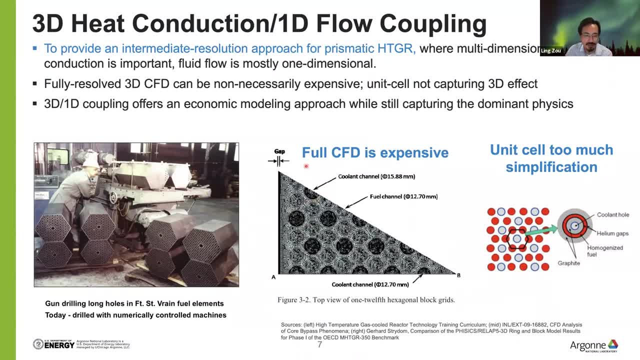 This is exactly happening On the slide, I mean on this plot. you can see, actually you have far more meshes is used in coolant channel compared to this, like heat conduction in this fuel pellet fuel rods. The reason is that heat conduction 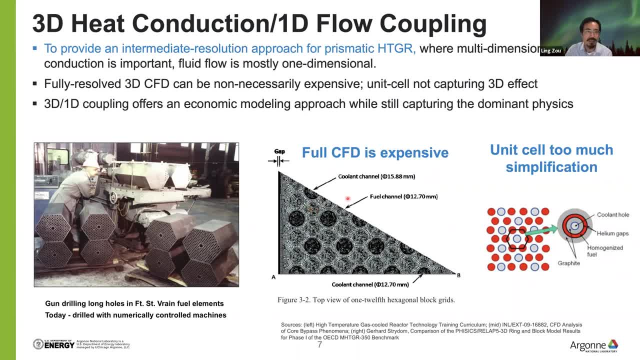 you can use quite relatively coarse mesh. So we can see that if we want to get a little bit more resolution compared to this like a system level application in so-called the unit cell. So basically the unit cell is like you just pick out one coolant channel. 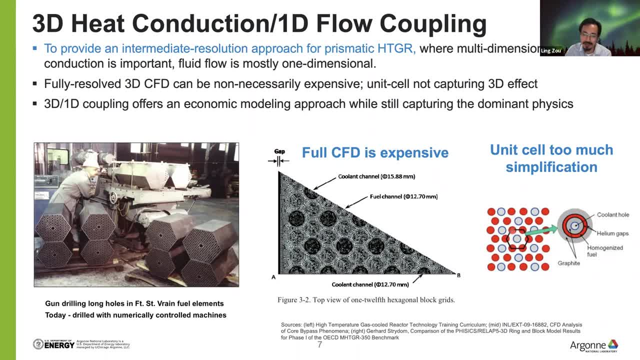 and then also use the surrounding fuel rods and then making them into this kind of like a ring shape. So basically you give a little bit of distortion in the geometries but trying to simplify the simulation, So you can do this kind of system level simplification. 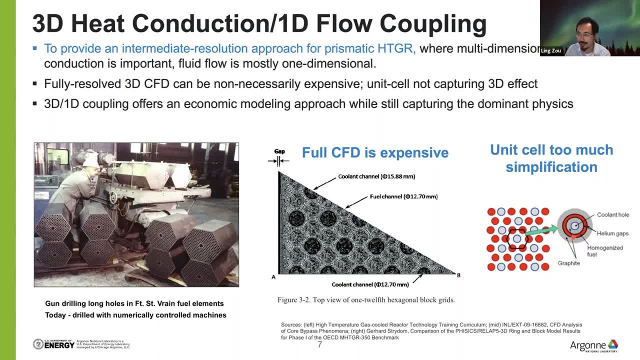 but you can definitely already tell the disadvantage of using this type of approach. You can just use one and then this one just representing a fuel block, and it shows some kind of like average behavior. But if you want to have higher resolution then you have to go to for CFD. 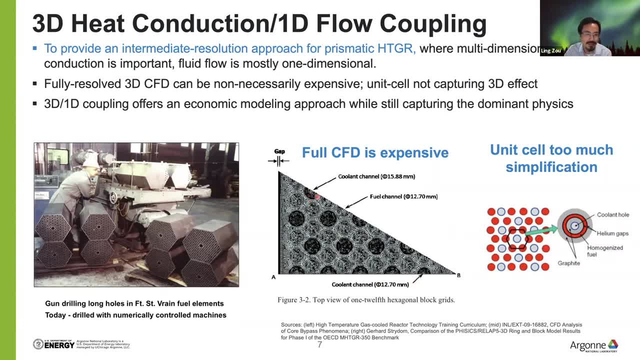 and then we just mentioned that using for CFD, we are wasting a lot of mesh in this coolant channel. So we are looking, actually based on this existing capability, We say, okay, we really need some kind of economical way to do that. 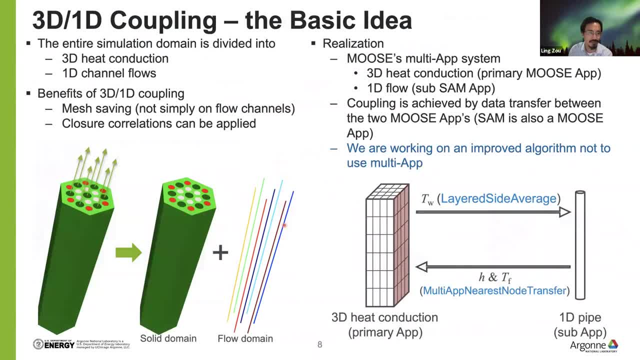 So this is. we have developed this so-called 3D- 1D coupling. So the basic idea is that we do have a mesh for the solid structure, but we don't mesh the flow channel, But just using this like 1D flow channel to model this flow. 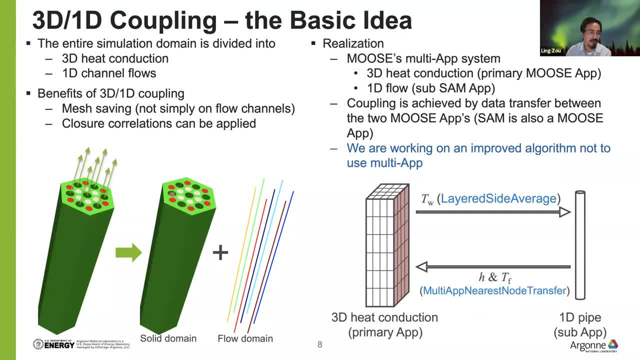 So basically, you can save a lot of mesh in this solid domain. It's not just that you remove the mesh in for this coolant channels, And also because you do not really let me go back, because you really do not put a lot of 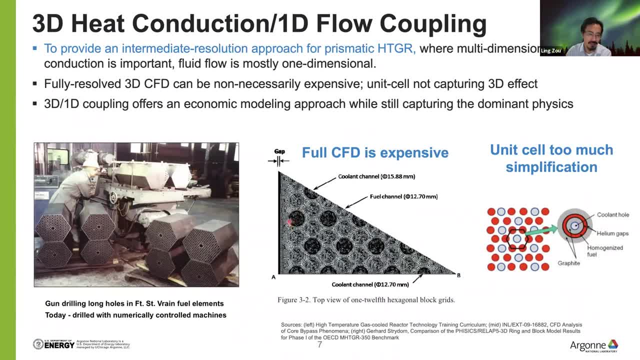 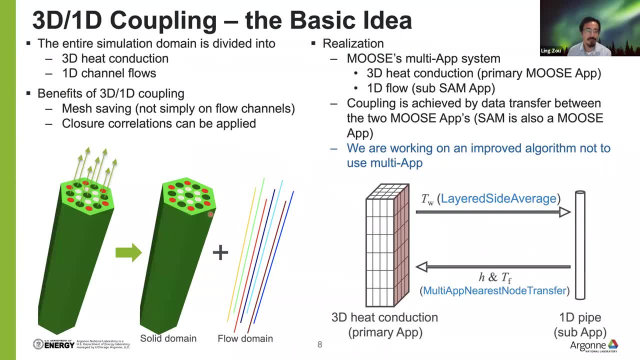 you know meshing here, then you can actually make the mesh coarser in this region. So there's a there's a big saving in the, in the meshing And then, but we still we are able to capture the dominant physics. 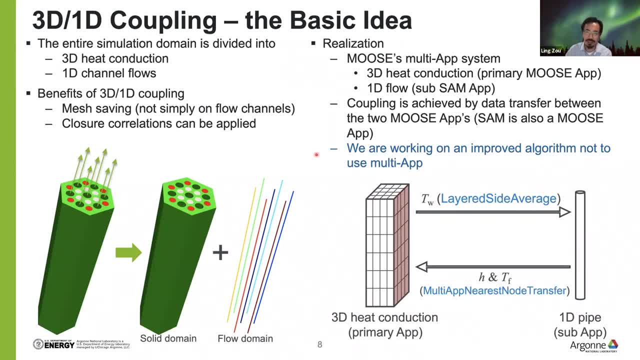 So the realization is based on the Moose multi-app system. We're not going to talk about how we do that, but basically there's like some data transfer between these two apps And then actually recently, we are also working continuously to working to improve this algorithm. 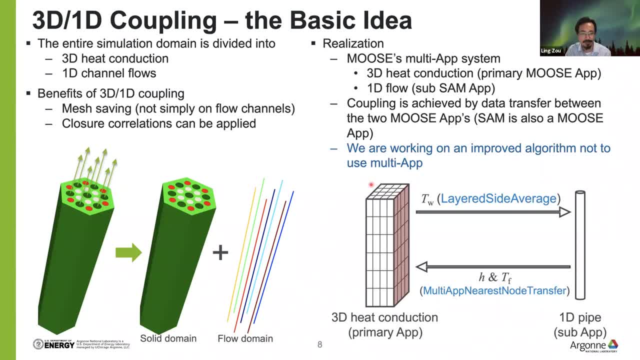 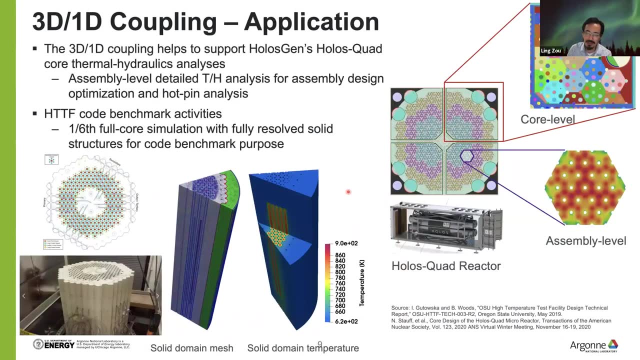 So the purpose is not even to use a multi-app. we can model the entire thing in a single application. I mean single application here, I mean Moose application. So on the next slide just several examples that how we use this intermediate resolution capability to help us in different applications. 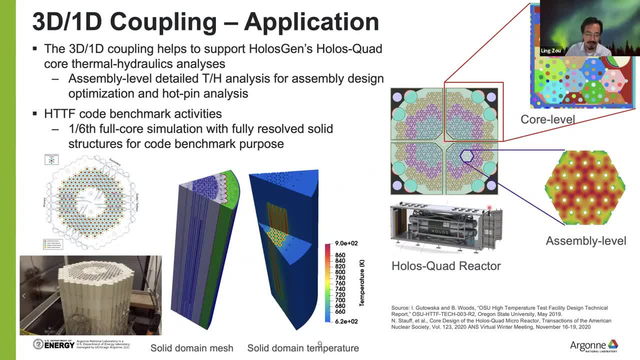 So, on the right, we have this Hollis project. As I mentioned, we are supporting HollisGen to design their so-called Hollis-Cord Hollis-Cord reactor design. So basically we can use. if you look at here, 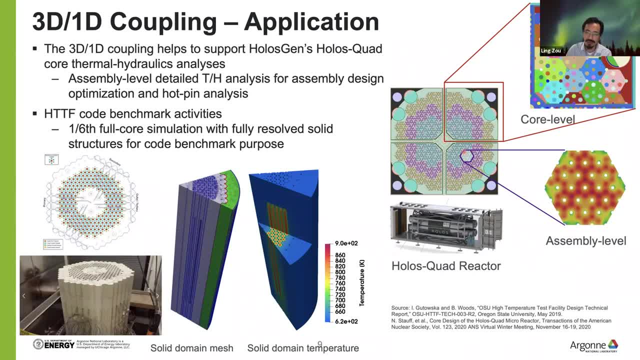 we can do some assembly level assimilation, focusing one assembly. Actually, we can do all the assemblies And so we use this capability to help us to have a better design for the assembly. So you can, you can totally see that if you are using the unit cell approach. 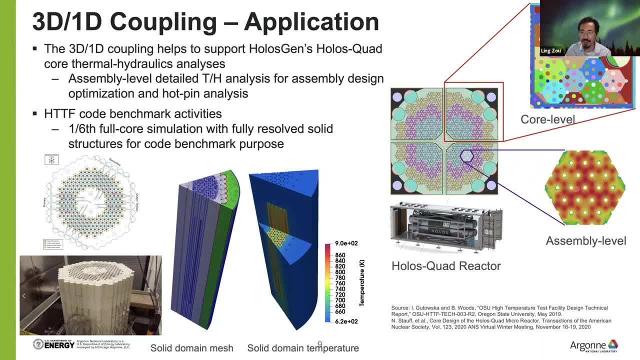 you cannot have this kind of resolution. You will only have like one, one representative cell for this entire field assembly. So we are not using that. We are not able to capture such a resolution because we we sometimes we need such a resolution for the design and to couple with the reactor physics codes. 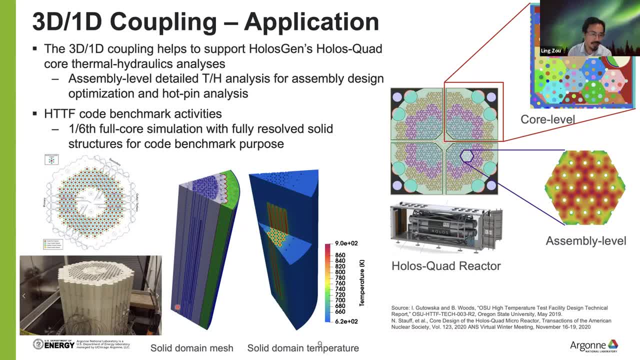 Here's another example is for the HTTF code: benchmark activities. HTTF is a scaled down tested facility at Oregon State for MHTGL, which is a GA design. So you can see that we can really model the entire reactor, not the reactor. 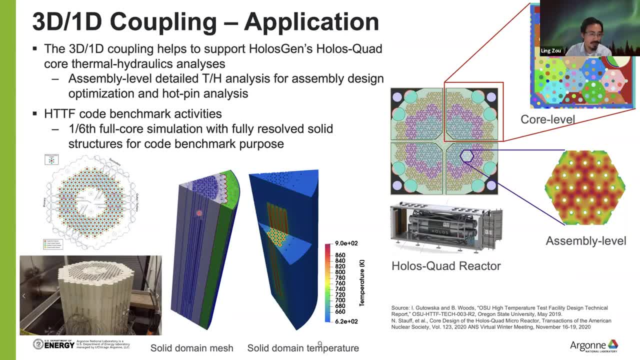 I mean this facility, the core region, and then we can model the solid part and then using the 1D to to model this, like the coolant channels, And then we are able to run the simulation. you know, very reasonable time. 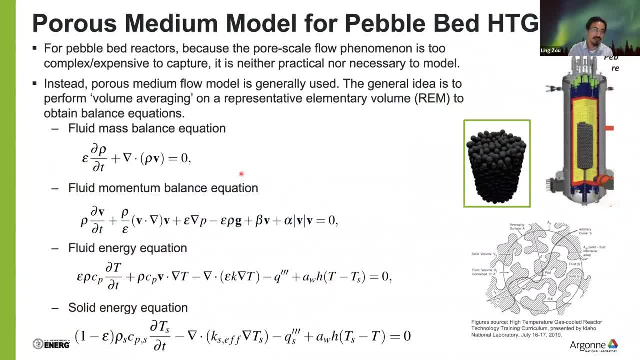 So this is another topic I'm going to talk about, which is the, the proximity model for the paperback, the HTTF. So, for the paperback, the reactors, because the, the poor scale flow phenomena, is very complex And if you want to fully capture them using CFD, 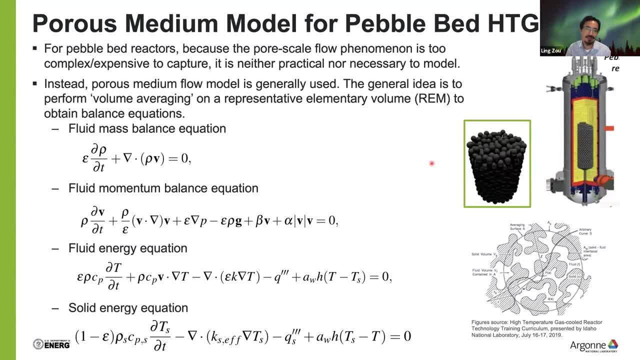 it's going to be very expensive And, from engineering, scaling is normally actually not necessary. Instead, we use so-called the proximity flow model to to model the flow behavior in the paperback reactor. So the basic idea is just to to perform so-called the volume averaging. 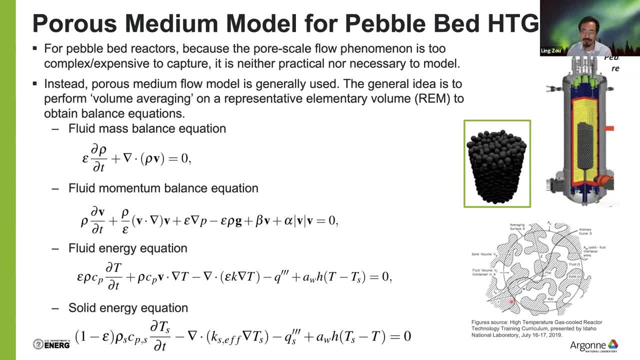 So on a representative elementary volume. So basically, if you in a simplified plot you can, you can see this is the volume we we have and then we do the average of the, the small scale equation, and then get to the average equation. 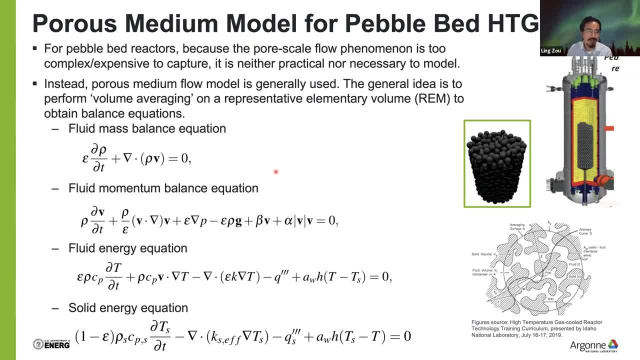 So basically, normally we will have the, the fluid equation, which has the mass balance, momentum balance, and then also the energy equation for the, for the fluid phase, Because of the, the solid. that also is a part of the domain that we. 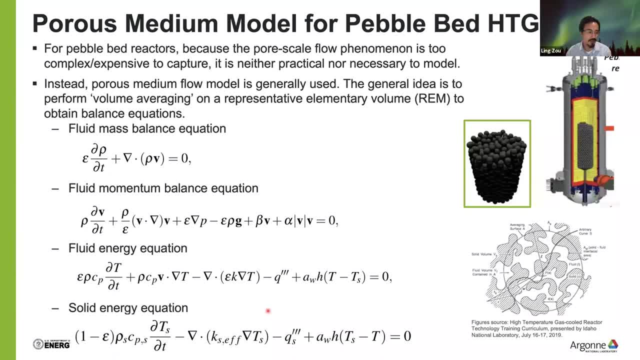 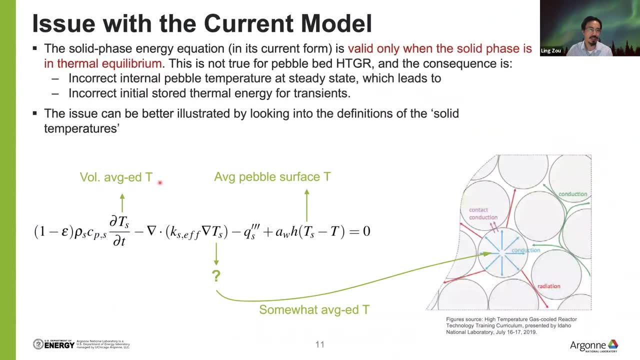 we want to capture is temperature, is heat source. We would normally have the solid energy equation for the, for the pebbles. So this is the, the baseline, all the very popular model we have. but actually there's some issue with the current model. 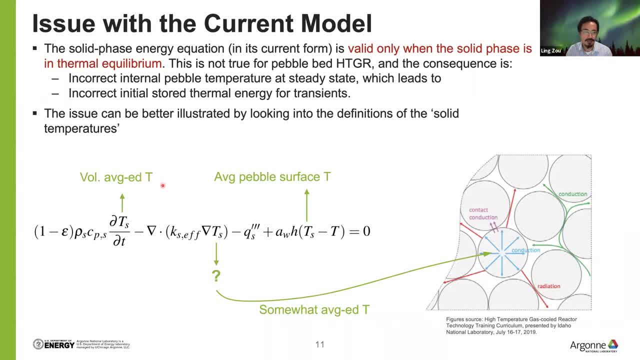 which is the solid phase energy equation. What do we notice? that is, that this solid energy equation is only is valid only when the solid phase is in the thermal equilibrium status. We know this is not the true for our pebble bed, HTGR. 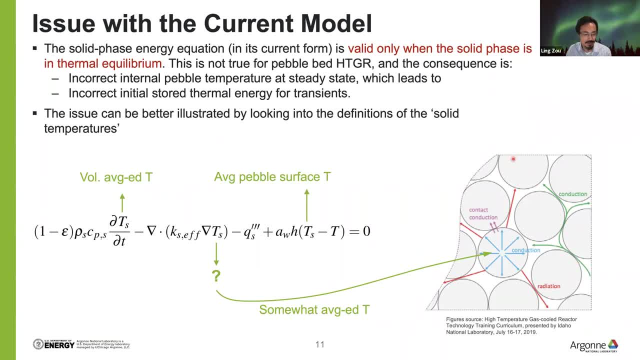 because we have all the pebbles there. they're hot. All the energy, all the heat sources, they are within the pebbles, all the trisoparticles. So if we're using the same model, then we are going to have an incorrect internal pebble. 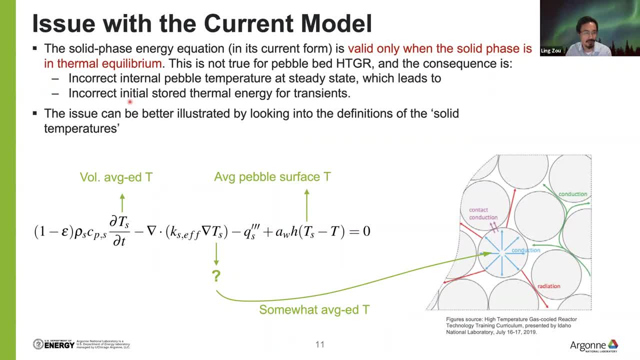 temperatures at the steady state, which leads to an incorrect initial stored thermal energy for transient. So you know, unless you will not be happy about that, because this is definitely a non-conservative assumption for them to use. So we can, we can look into a little bit more details to. 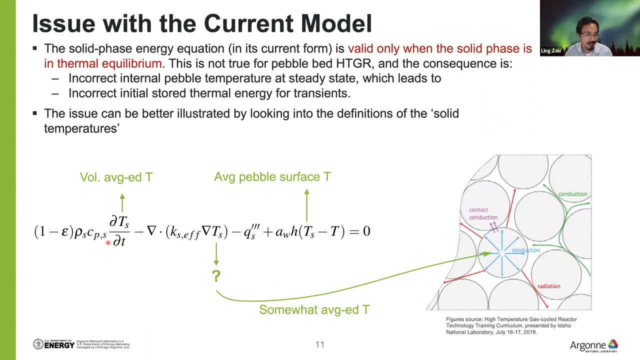 to see why it's the case. We can look at the average temperature or the temperatures of this solid temperature. The first one, the transient term. we can totally see that this is associated with the volume average of the solid temperature. But this 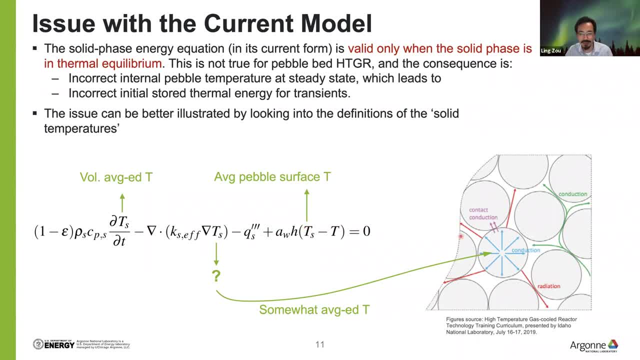 the convective term is this: solid temperature is actually the surface temperature or some some sort of like average average surface temperature. And then this another term accounts for the, the pebble to pebble heat transfer. It's it's very complex here. 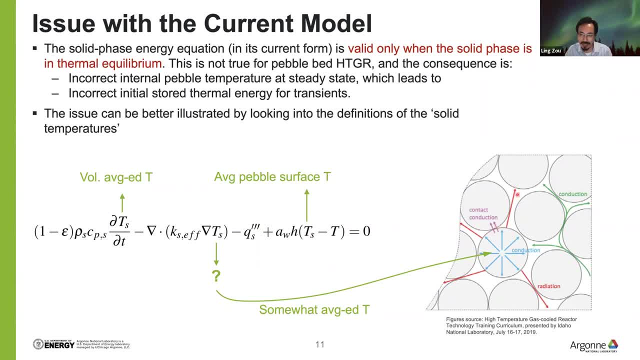 They. we have like a contact conduction. we have a thermal radiation, we have a conduction through the pebbles and then we have a conduction through the, the gas phase, and then and then to the, to the another pebble. 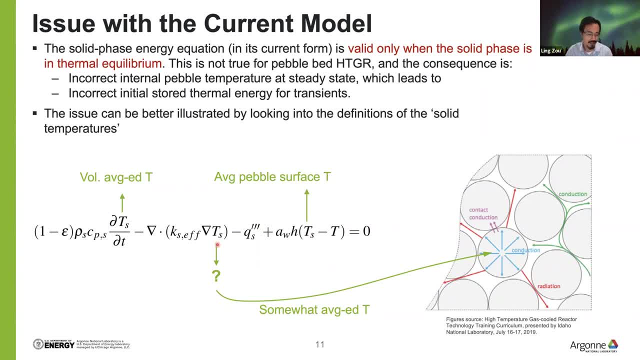 So so actually you can, you can tell this: solid temperature here is kind of like a mixed definition. It's it's neither volume, it's neither surface. it has some kind of like a a mixed definition here. So actually from the literature: 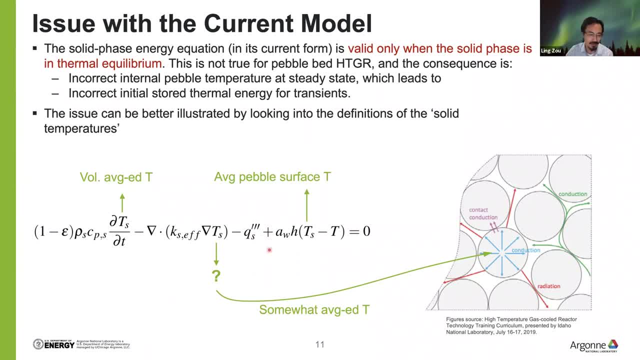 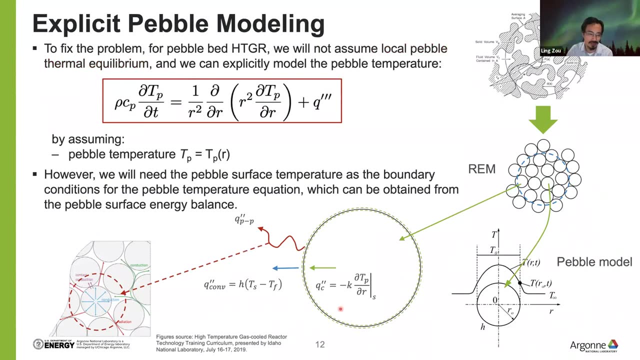 I've never really seen how how this temperature has been appropriately defined, But anyhow. anyhow, I think that this already explains why this equation has some issue. So, in order to capture the pebble behavior during both the transient and the normal operating conditions, 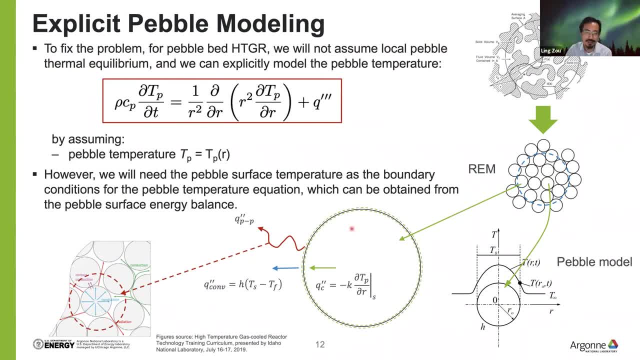 we want to explicitly model this pebble. So if we look at the, the elementary volume, the volume of this pebble bed, we can see in each of this like a representative element or elementary volume. we can assume this: the size is big enough to contain several pebbles. 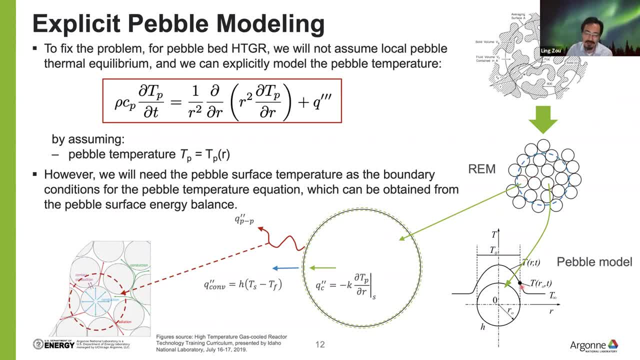 And then in each of this volume we say we have a representative pebble which is here It's. you know, it's like representing the average behavior of the pebbles in this, like a bigger volume. So basically, yeah, 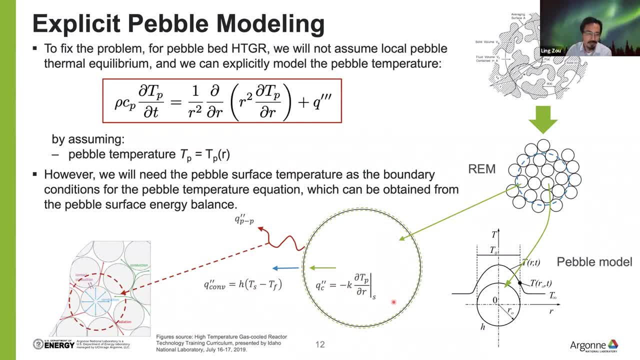 we know it's. it's actually kind of easy to model a pebble, If we can assume that is we using the 1D spherical coordinates. we do not model the. you know the, the, the difference on this wall. 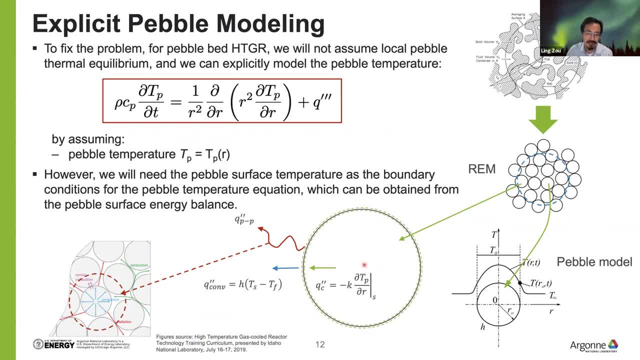 but we assume on average it behaves like just the 1D behavior. So we can model it with the 1D heat conduction model in the spherical coordinates coordinate very easily And we have everything we need. The only thing we are missing is actually the surface temperature of this pebble bed. 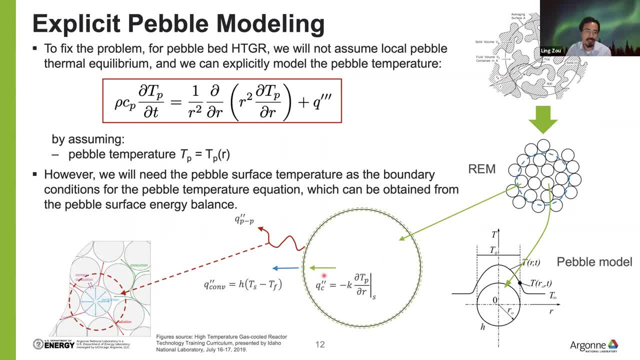 pebble And the surface temperature can actually can be obtained by the, the energy balance through this infinite small layer. So basically, we have a heat conduction within the within the pebble, And also we have the, this heat conduction through the. 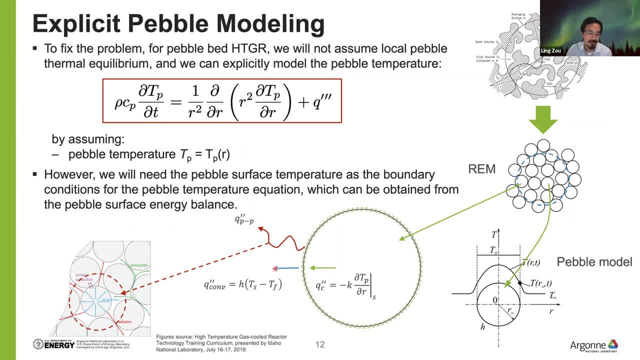 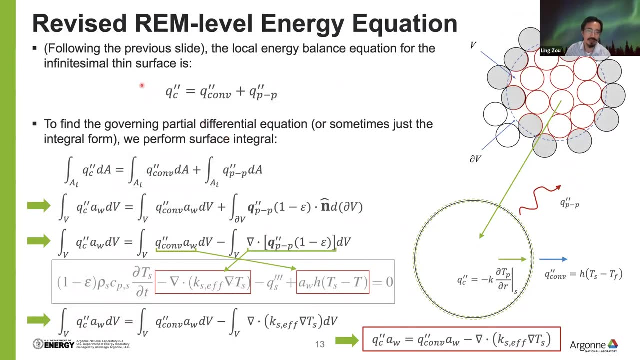 sorry- heat convection to the, to the fluid phase, And then also we have this pebble to pebble heat transfer, which captures all the same complex mechanism. So, following the previous slides, we have this balance equation, but this isn't just a description. 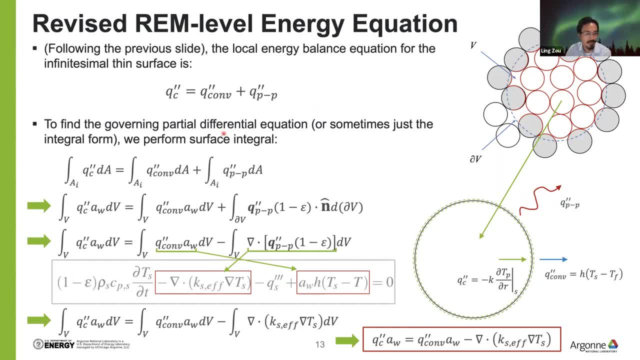 We need to transfer or to derive the the governing partial differential equation, or sometimes we can just use the integral form. So we perform a surface integral of this equation on on this surface, not on this just on the surface, but on all the surface in. 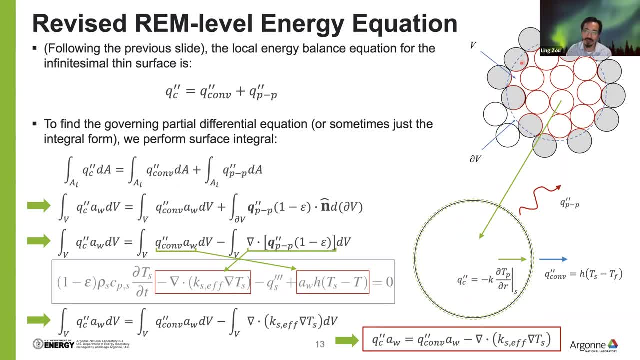 with inside of this volume. this is our representative volume. I'm not going to do all this math here, but there's quite some math involved. You will have this like: from surface to volume, integral, and then you you have to apply the divergency theory of the Gaussian theorem. 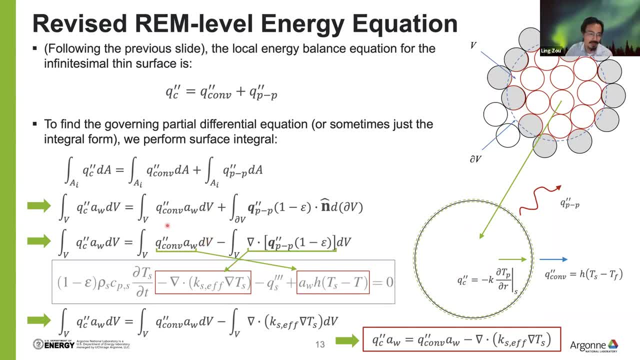 twice And then eventually you can associate some of this for them, the convection term, into this original conversion convection term in the original, the older model. And then we were associated with this pebble to pebble heat transfer, associated with 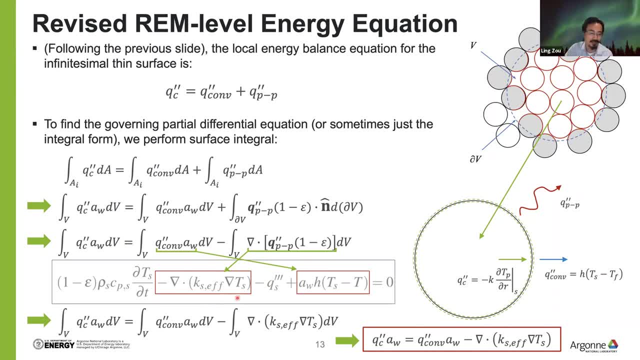 to this original so-called effective heat conduction term, But then eventually we arrived to this, the PDE form, or for this energy balance in this infinitely small surface. So, basically, the idea here is that this is the original model. You can see that this model has been split. 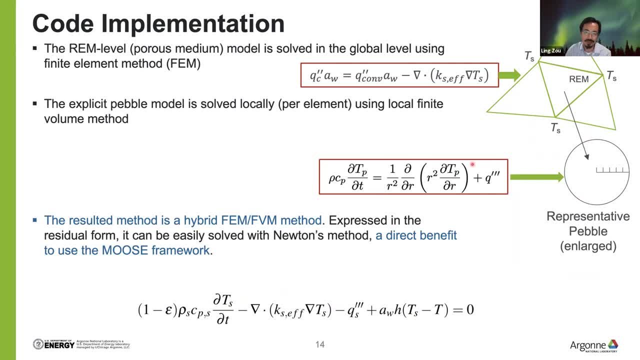 split into these two models. One is the pebble, better explicit pebble model. This term is the the time dependent term, which is when you average this guy, you get this term, And then this is the additional spatial term within this pebble. 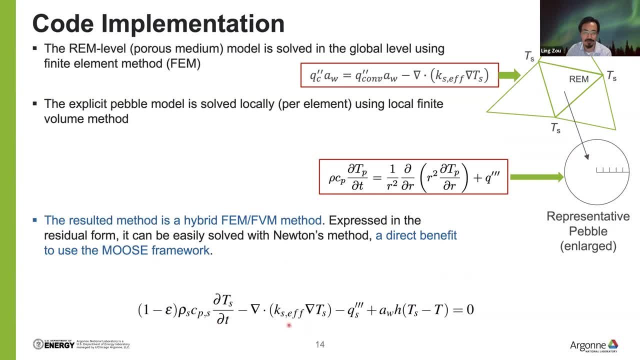 which you, you do not capture in this term because you, you perform an average already. Then this is the heat source term, which is, which is this term, And then you can see that some of these two terms, they go into this to. 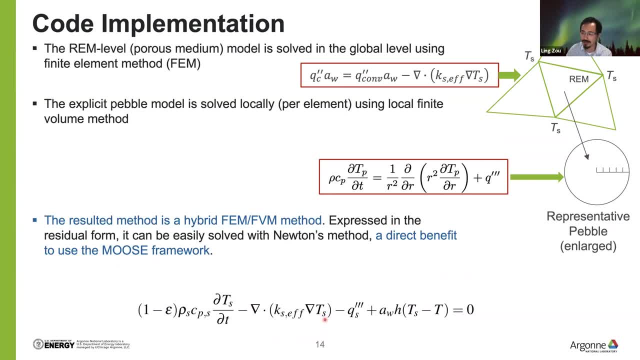 in this equation, for example, this effective pebble bed heat conduction term goes into this term, And then this convection term is this term, And then you see, this additional term is actually a, a bridge or a connection term into this term. 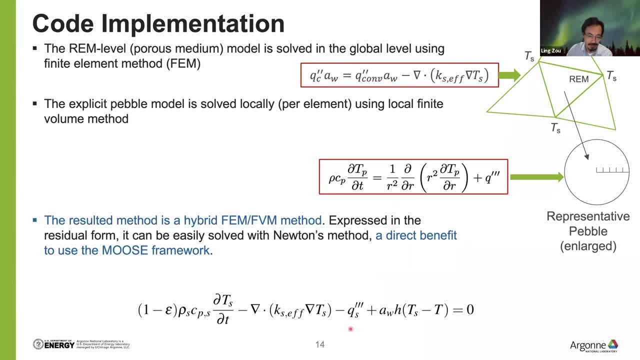 which is spatial there. So, basically, idea, we are split to the original equation into two, four, into two equations And then with added resolution we can capture the pebble internal temperature distribution. So the implementation, we put it in the Moose framework. 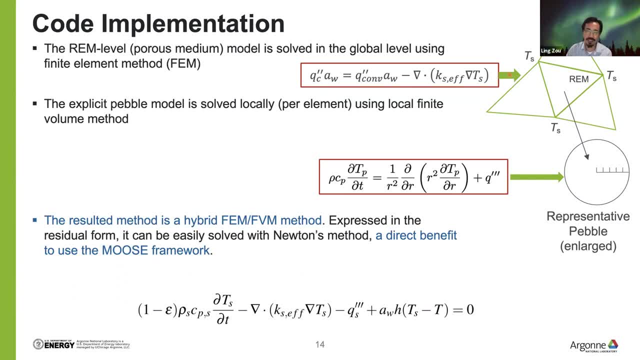 And basically this term represents the, the IEM, or the representative elementary volume. So it leaves on this like a global mesh. And then this pebble bed, sorry, the pebble, the explicit pebble equation they leave within this element. 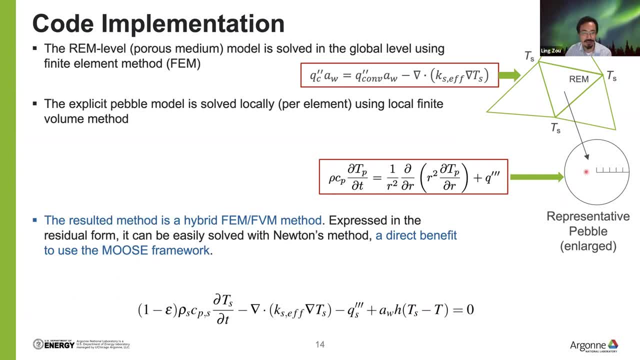 So it has these local coordinates. So using Moose, we are able to solve this, the system, very easily. I mean, this cannot be easily done if we are using other type of a technique, And so this is really a direct benefit to use the Moose framework. 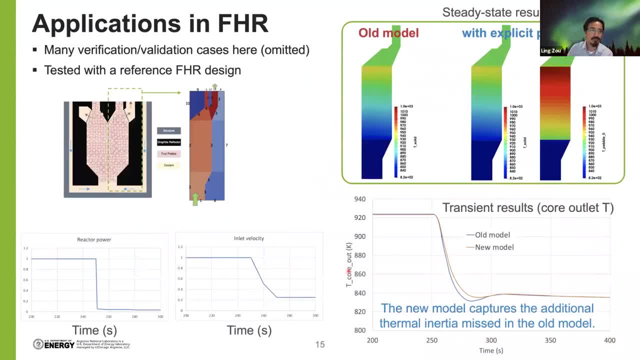 So here I'm going to probably talk a little bit about the application. So we did a lot of verification, the validation case of this newly developed capability, but I'm not going to talk about the here. So you know all this: verifications. 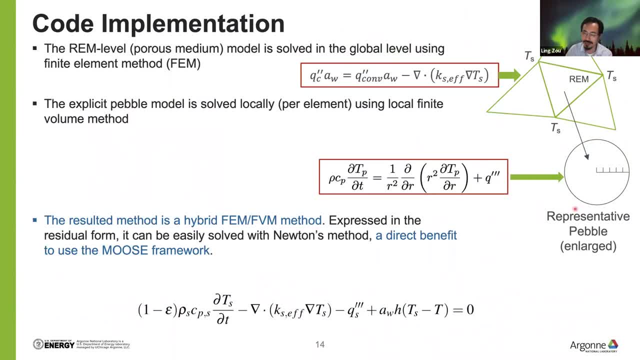 they're really. if we go back here and you have a lot of like how your temperature should behave when you have like internal heat source, when you have some boundary condition and sometimes you have like your pebble bed, I'm sorry. 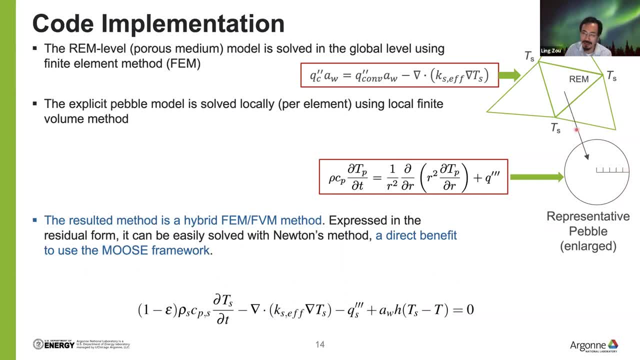 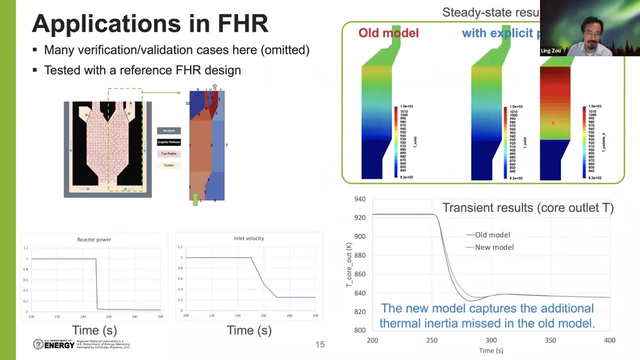 pebbles, you can assume they are suddenly got a cranched into this like a bigger volume with, say, coolant. And then we have a lot of cases like doing that to to make sure that the code implemented has been correct. So after all this, 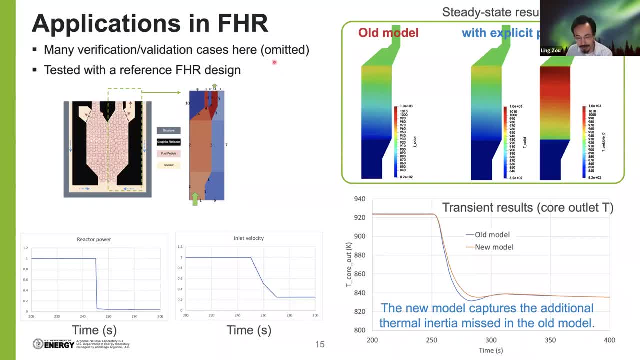 like a verification and the validation case. we would like to look into a more, more or less like a demonstration case in the FHR design. This is what the NRC. they are interested. you know they are interacting with some industrial companies. 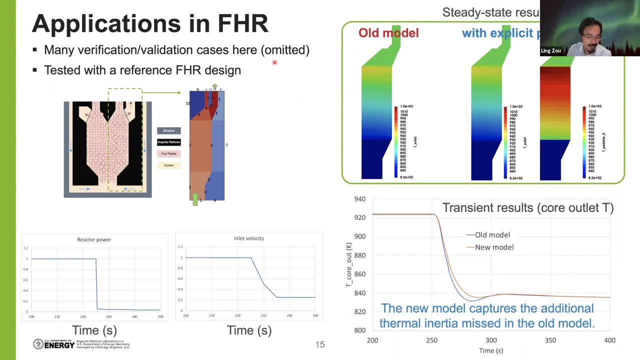 you know doing FHR designs, And they want to see how the, the code, can be used to predict the chance and behavior of the, for example, FHR or HTGR. So here we have a reference design and you have this. 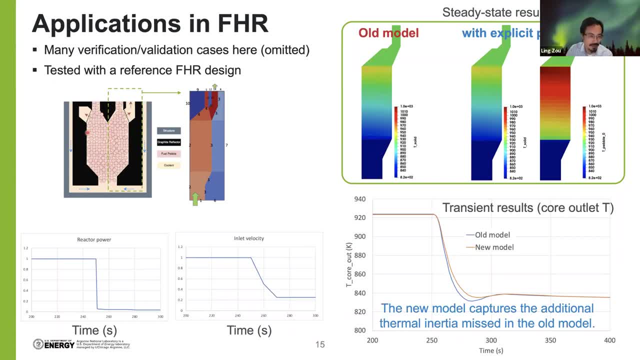 like a pebble bed, that we take advantage of this like a cylindrical shape of the reactor. So we are using the two dimensional RZ geometry to represent the, the core. So basically, the red part is have the their pebble bed. 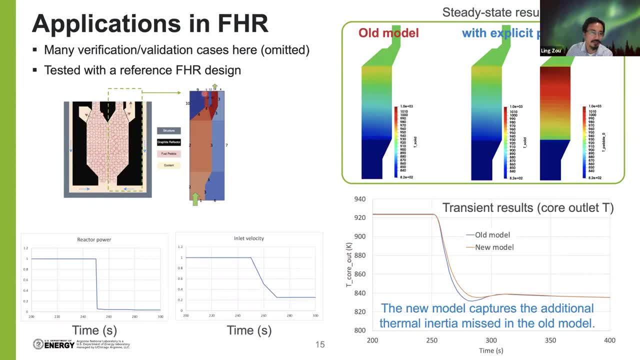 This is a dead zone because there's the pebble is not moving, The flow is not moving too much, And then this is active core. Here we have demonstrated a pump trip scenario. So basically, your, your net velocity is like dropping down from one and then down to some value. 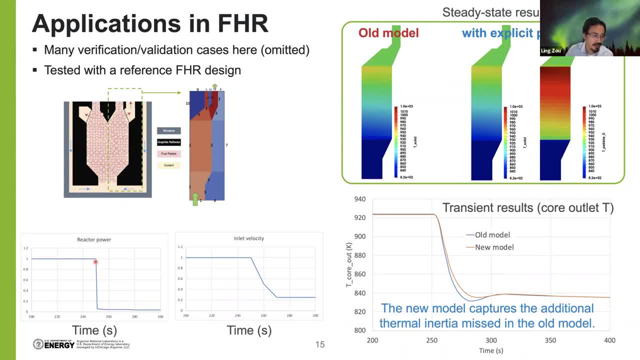 And then your reactor scrams. So your then you go to into this like a decay heat mode And here's some, some results in the in the old model or the original model, as I said, that the solid, the temperature is really only represented the pebble surface temperature. 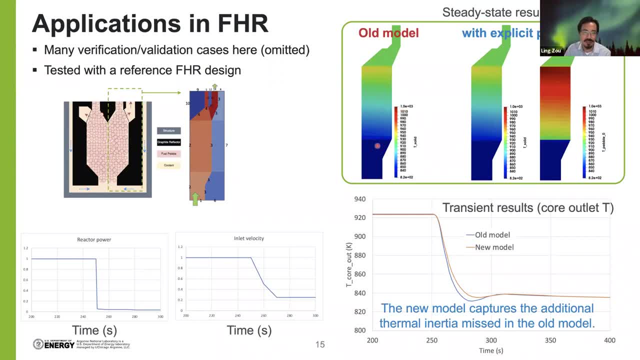 So here you. we only have one temperature for the solid, which you really just that, the surface temperature. But if you look at the new model with this explicit, the pebble model, we have actually multiple temperatures. So one here is still the T solid. 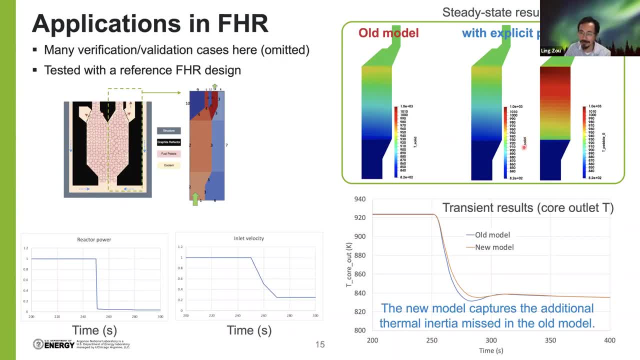 Now the T solid is really representing the, the pebble surface temperature. And then we have this T pebble bed, T pebble zero. Here zero means the, the very, you know, the, the, the inner layer of the pebble. 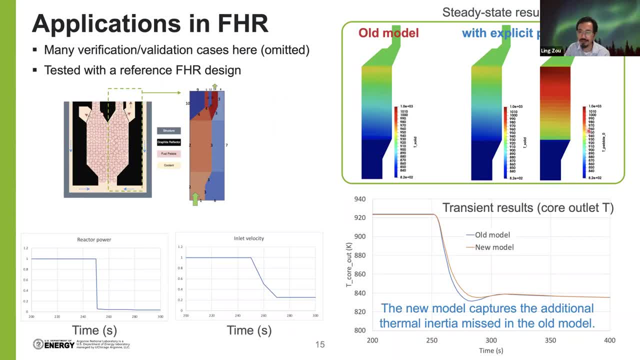 or in other way: this is the pebble center temperature. We can see that these two temperatures they actually they differ very, quite a lot. I think here we are not not so sure the scale here, I think probably in the hundred degrees C level. 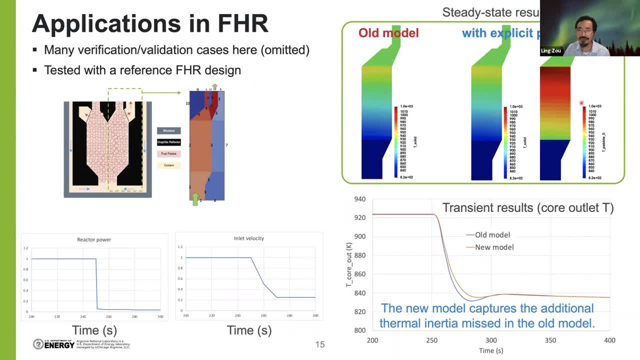 not, not so sure, but you can see the temperature is different And that put it in another way. in the older model, all the solid, the temperature is in the same temperature of the surface temperature, And then in this new model we are able to capture the temperature within the pebble. 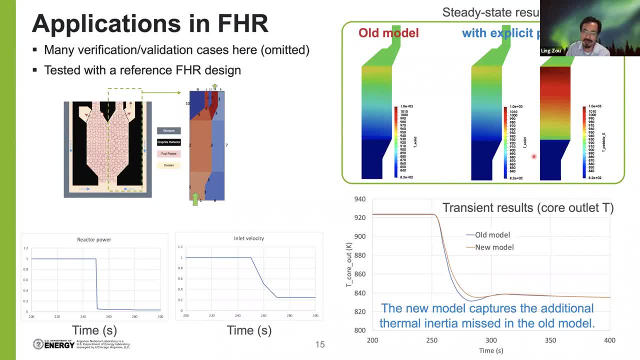 So we are able to capture this like additional thermal store. the thermal energy in this pebbles. So if you look at the chance and the results, look at the core outlet temperature, which is the fluid temperature and the outlet, you can see this new model is actually. 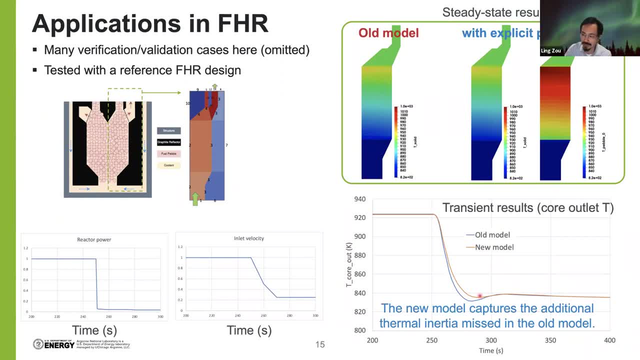 is higher than the what has been predicted with the older model. So you know, the difference is not big about the say somewhere like a 10 degrees C, but this, you know, NSE is concerned about this type of behavior that if we use in this, 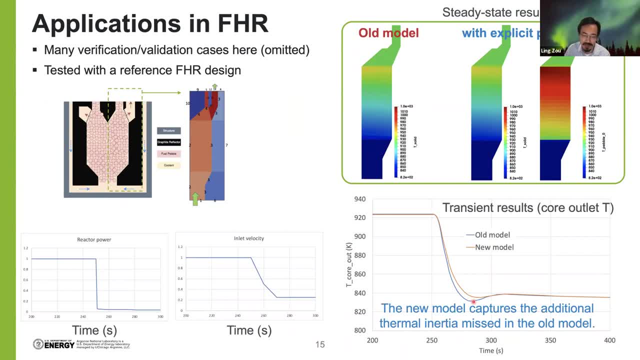 older model is really represent a non-conservative assumption. So this is for this work. as you see, we have some theoretical derivation and also we have some coding implementation, which is the Moose framework. make it flexible, but we want to emphasize that the 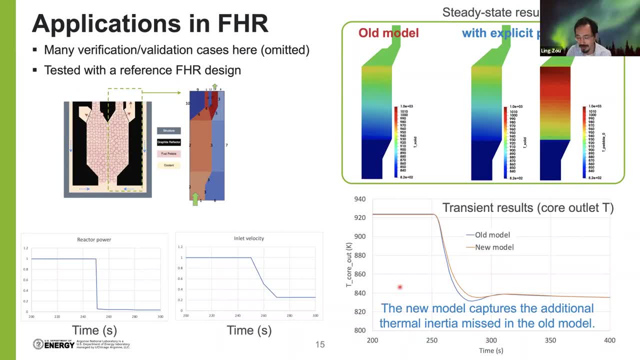 in, for example, in other, in the traditional way. if you want to implement the code, normally you are going to do it in a quasi quasi-state state way And this is actually typically seen in the in the older codes. 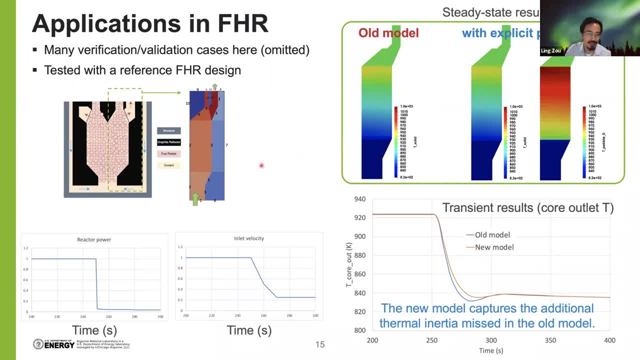 in the existing literatures. Basically you you have to come compute the surface temperature, then you do the back calculation for the pebbles. So with this you know the Newton's method, or the in the residual form. 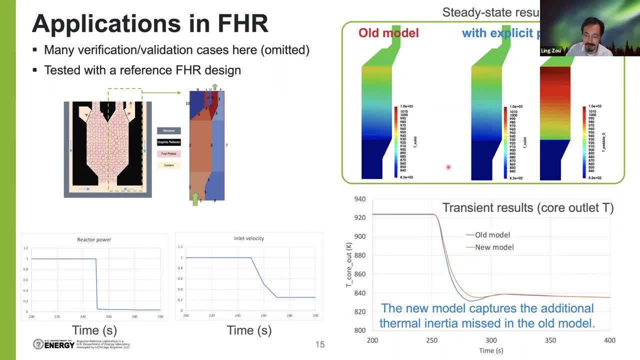 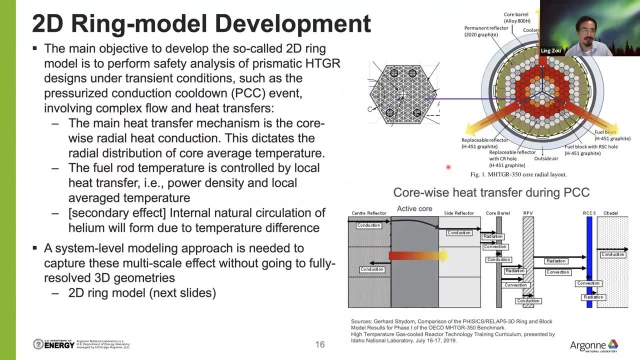 we can easily implement the cow then to demonstrate the time. So with this I'm going to change to the last the topic of so-called 2D Remodel development. So before I talk about how we do it, we want to give a little bit back dinheiro to explain why we need that. 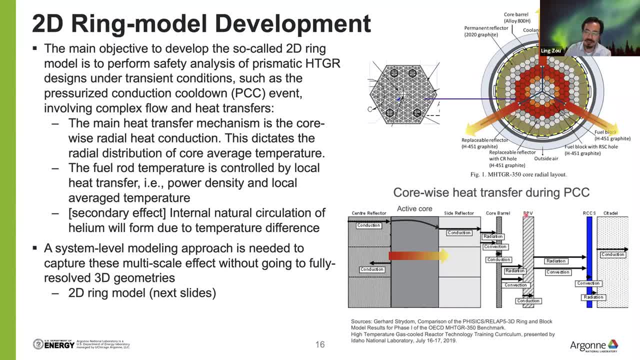 So so here is the how how to like the decay heat removal is happening in the freedom in the htgr. so i think i i talked a little bit about the rccs rccs system in the previous slide. so if we look at, look closely, so normally during 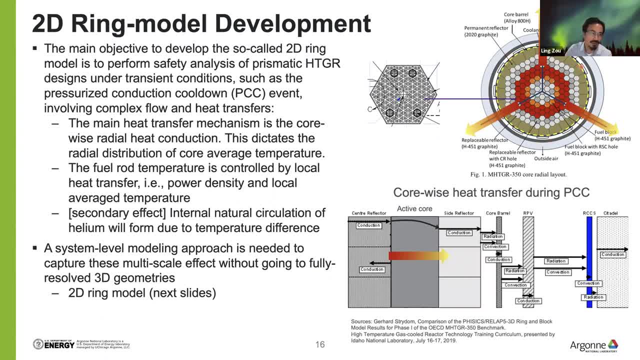 the freedom, a so-called the pcc event or pressurize the conduction, cooling, cooldown event. so basically, you don't have your external power, so your helium blower does not work anymore. and then now you have to remove your decay heat. so your decay heat removal path is actually from the 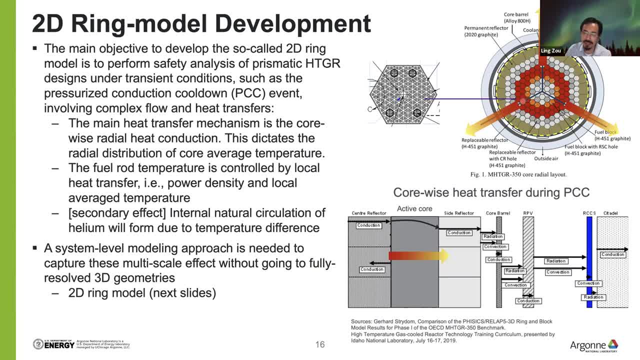 core and then it goes to radially through this like a reflector and then it goes to the core- i'm sorry, the- the reactor vessel and then eventually the. from this uh reactor vessel it goes to the rccs cooling panel. so if you look at this um, this rz. 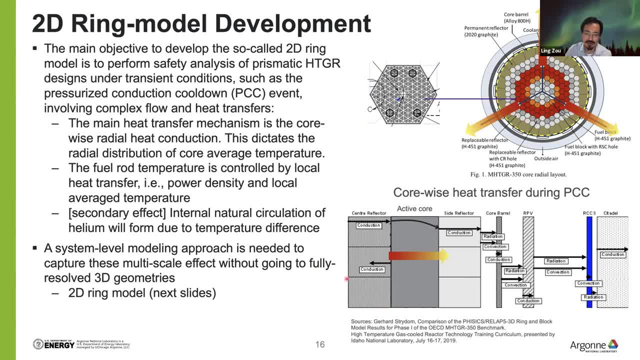 direction, it probably will be clearer. so this is the, the center of the core, this is the center line, so this is center, with central reflector that does not have a heat source, but this is active core. even you, uh, squirm your reactor, you still have the decay here that you need to remove. and then 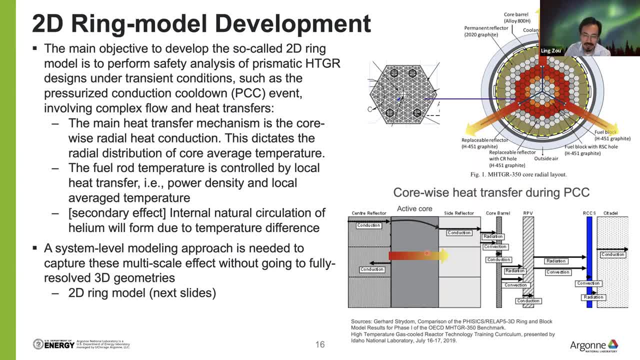 during the transient. so this cup becomes hot and then you have this like a radio heat conduction through this active core and then go into the, the reflector, and then we have some radiation to the core barrier and then also conduction radiation to the reactor vessel, which is which is here, and then it leaves from this. 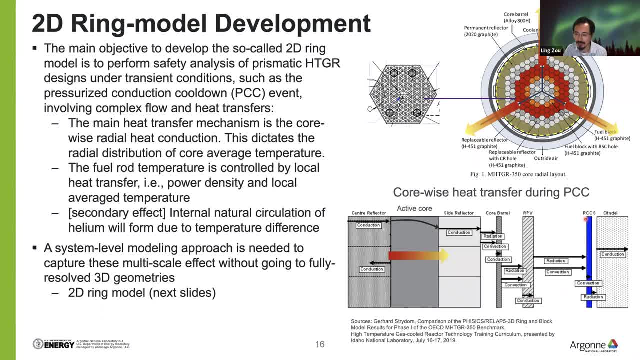 reactor vessel surface to the rccs cooling panel through radiation. and also sometimes it has this like: uh, internal convection helps a bit, but the the majority heat is there through the radiation. so this is rcss cooling panel, so you can see that, um, i mean, this is the ultimate heat sink and you. 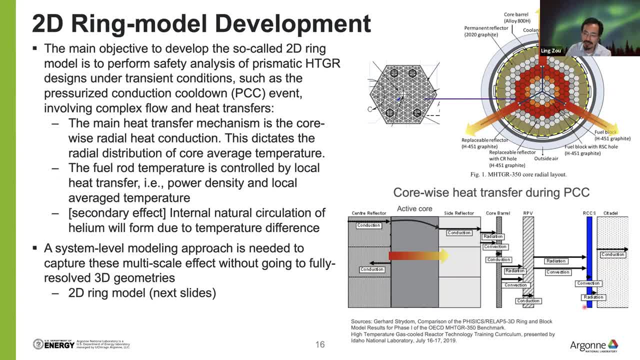 can see that if you go back, trace back, this is actually the anchor point of your entire system. this is the provider temperature boundary condition. then, if you trace back, you will notice that your entire core, or the average core temperature, is dictated by this core. wise heat conduction- uh thermal radiation convection. 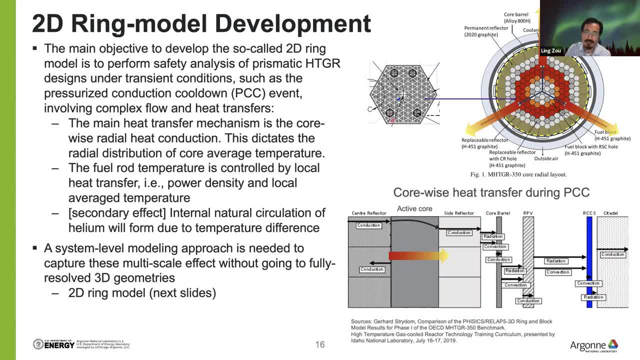 and if now, if you look at this localized fuel assembly, then when your average, the core temperature, is dictated by this bigger behavior, i mean larger scale phenomena, then your local fuel fuel temperature is dictated by your local uh heat conduction. you have a fuel pellet which you have an internal heat source, and then it talks to this um, averaged um. 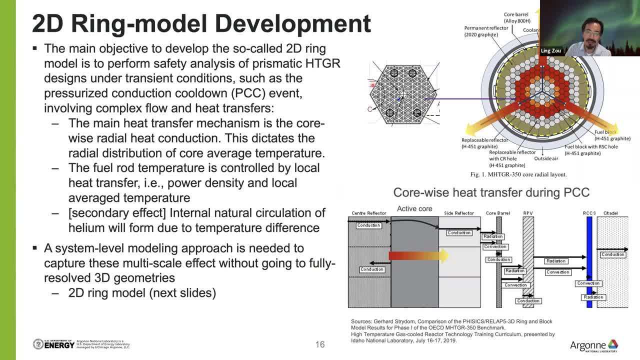 uh, solid temperature. so both of this scale they are very important for us to capture, to to get the peaking temperature and of course you can go to the full cfd. you know that's going to be very expensive and so the the main purpose here is we want to develop a system level. 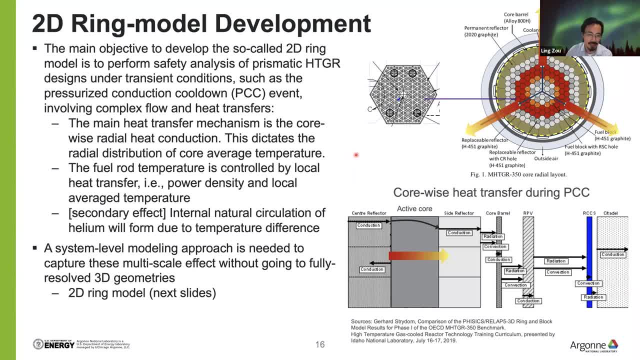 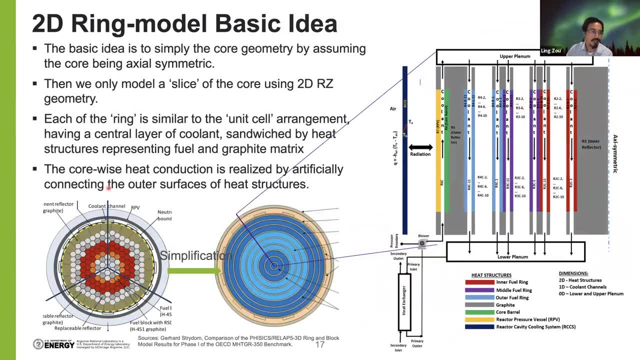 modern capability that is able to capture both um scales. so this is the so-called 2d remodel, which i'm going to talk in this next slide. so the basic idea is that to take advantage of this not so much like a perfectly excess metric, but we can say, okay, doing a little bit of massage to assume the um. 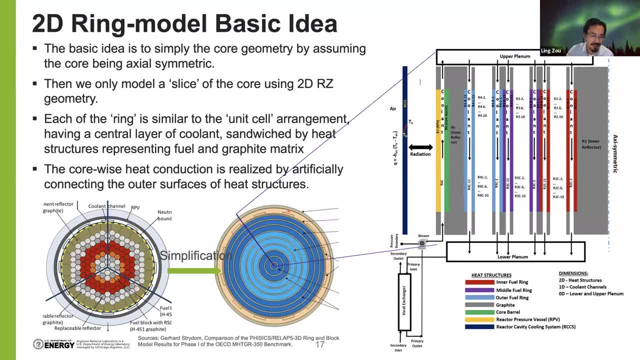 of this like excess matrix behavior and then transform it into this kind of like a ring-shaped one. now we have this like a perfect um excess match and then we can only model one slice using the rz and geometry to model a slice of this uh core which i'm i'm like showing up here. so 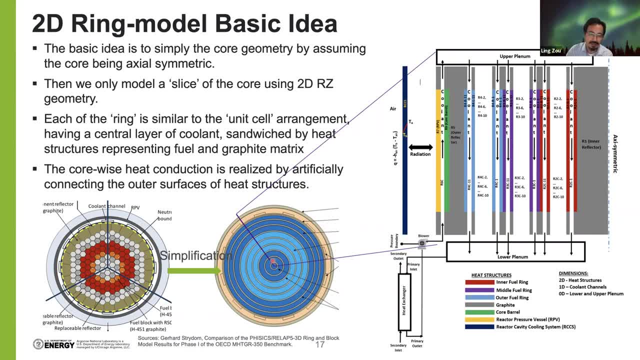 basically the idea is that, uh, we model this, um kind of put them in these layers of like graphic images, cooling the channel fuels and the cooling channels, feels this kind of configuration, and then each of these layers, we are kind of like a follow this, like a unit cell approach, and then, and between this unit cells, we are using some artificial heat. 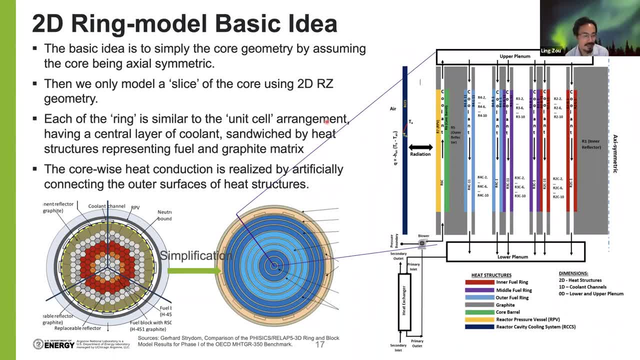 conduction. this can be done. that, i mean this is the beauty in the system level analysis. you can add, using this like artificial connection between the different blocks. normally you cannot do it in the cmd because you have to mesh them. so basically the idea is to use this kind of 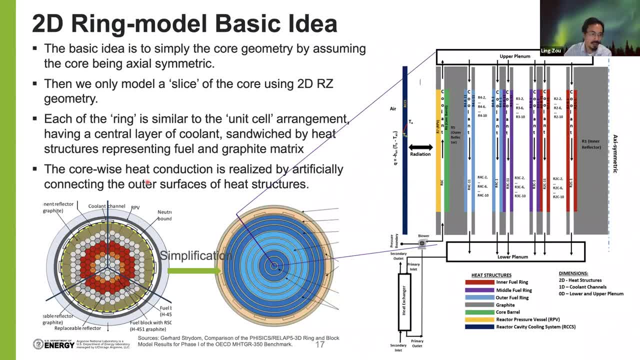 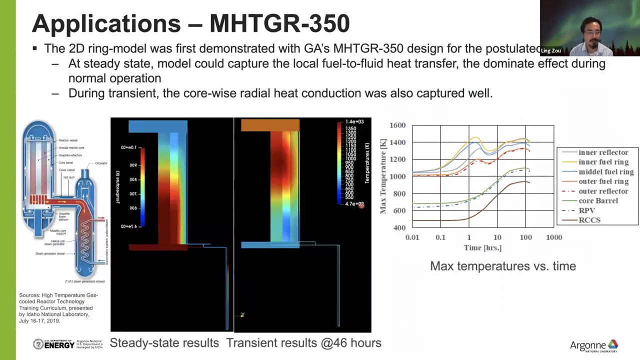 modeling approach to capture both the core wise behavior and also, with this kind of thing, to capture the localized hit, hit transfer or hit conduction behavior. um, let me see the slides are not moving. okay, that's moving. so, um, with this kind of uh modeling approach, we 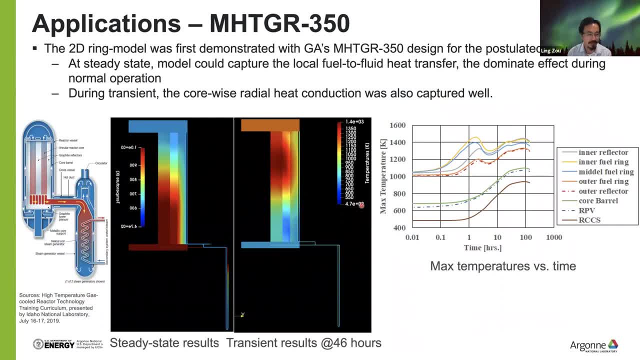 have tested this um modern approach using the htgr350, which is a ga design, and this is the general atomic design of the mhdj's prismatic design. so basically this is the core region and then this is the steam steam generator. so basically the flow is going from out of this uh coolant, uh big coolant channel, and then goes up. 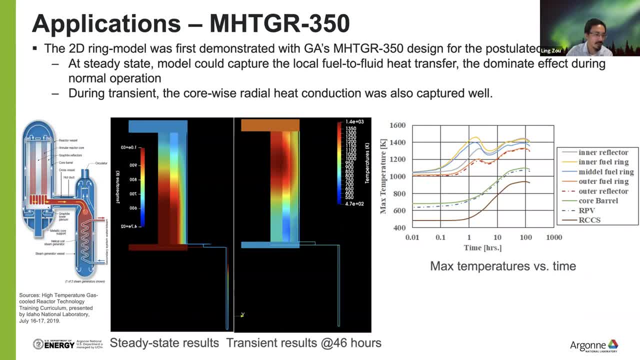 and then make a turn, going down and then going into the steam generator and then loses heat to the water and then going back. so this is the uh coolant, uh flow and the, and you can see that during the normal operating of the static state uh scenario we are able to capture such a um. 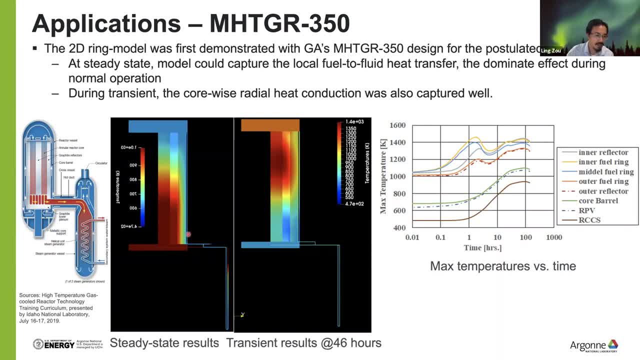 uh flow condition. you can see the simpson, the, the cool, cool, the cool and the going up and then make it turn and they're going down and then going: uh oh, sorry, it's going this way and then going back. so basically you can see, this is like: um, this is the. 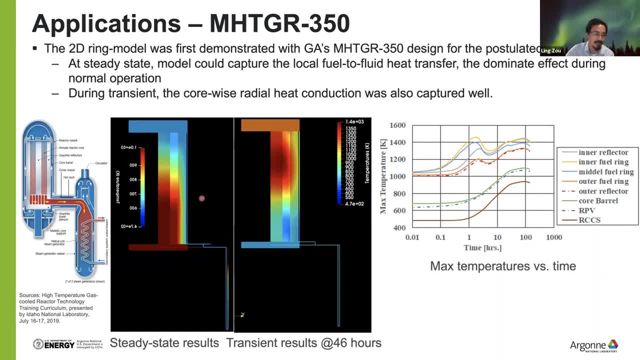 solid temperature is hot at the bottom because of the coolant going down. The coolant becomes hotter and hotter and then eventually. so this is hot to the side in your reactor during the static state, But during the transition, when you do not have any more of this coolant flow. 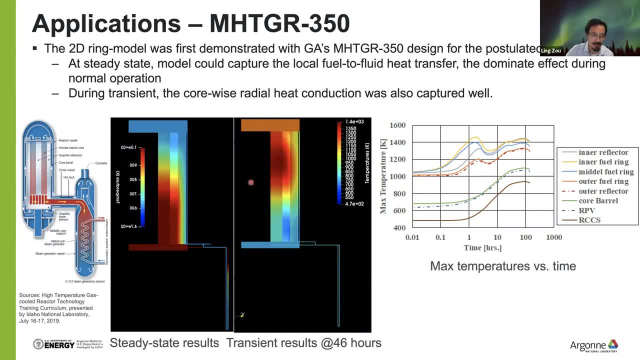 then the entire heat transfer becomes that, as I just mentioned, you rely on the radio core-wise heat conduction, And then the cooling panel is not showing here, And so the heat has to be radiated from the surface to the RCCS panel. 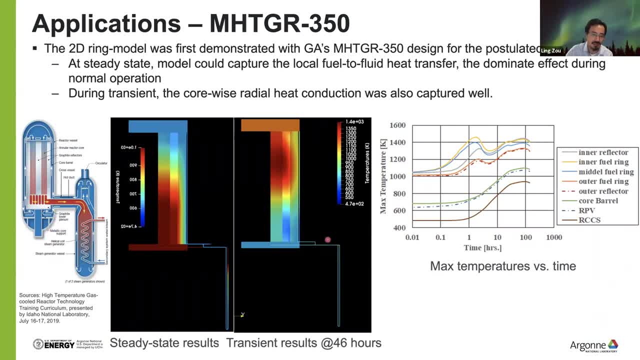 And then in the RCCS the coolant temperature in this case is: the air is also getting hotter and hotter and then leave the system. So the RCCS temperature is hot, here the air temperature And then also in combination with the cosine shape of the power. 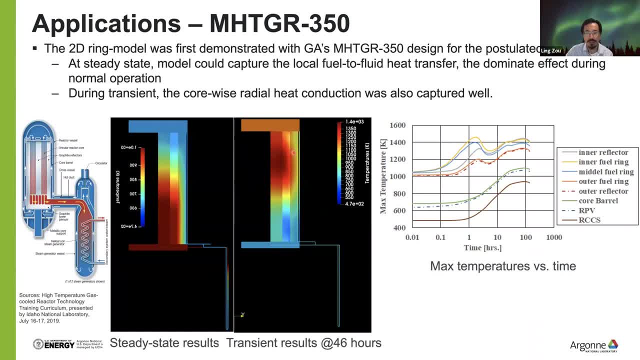 distribution. you can see that the hottest part is here. So basically, the idea is that the message I'm trying to say here is that this type of modeling approach is able to capture the local phenomenon during the static state and also is able to capture both the core-wise 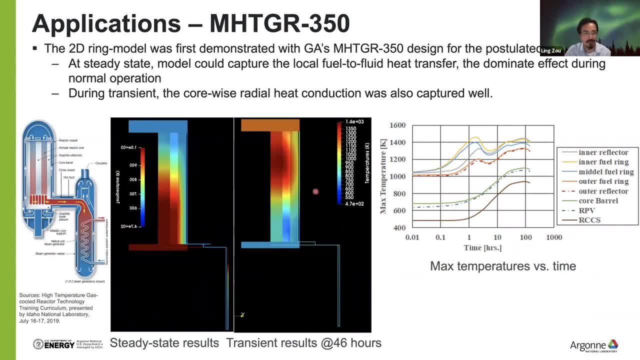 heat conduction and the summer radiation and also localize the heat conduction within this few blocks. So it's a very good approach to use for the prismatic HTGR. Otherwise, if we're going to the CFD, you may use the approach. media approach is also very time. 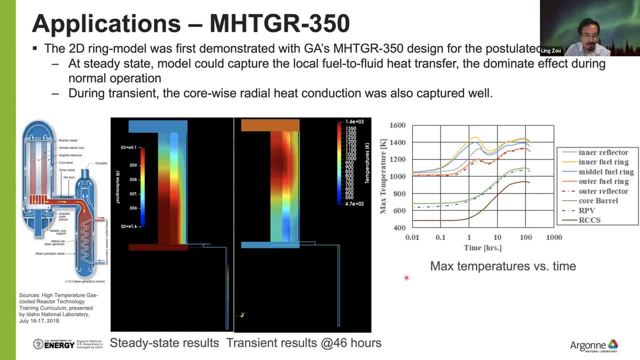 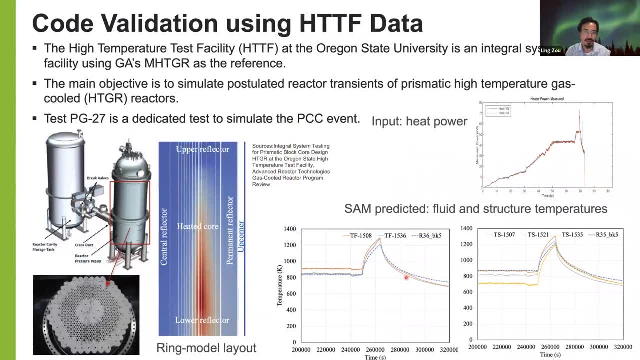 and also a lot of efforts to make them mesh. Another quick example is the code validation for the HTTF data. So the last slide shows kind of like demonstration. We developed this code capability. We want to see if it works, But we do not really know if it really. 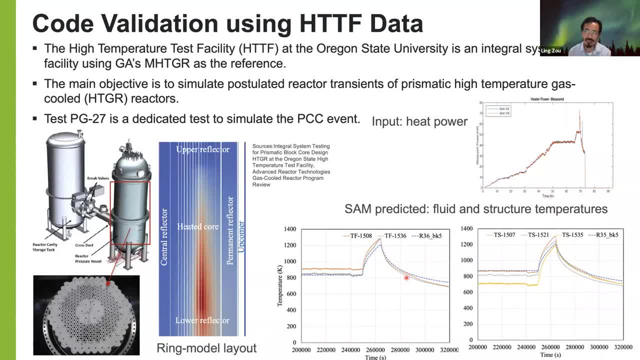 works compared to the reality. So, starting from last fiscal year, we start looking to the HTTF and then use it, Because they have this data we can use For code validation purpose. So if you look at the core, it's pretty much similar. 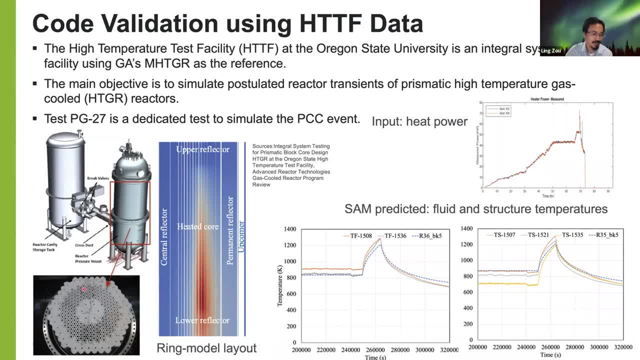 very similar to the MHTGR, of course, because this is a scaled down integral test facility for MHTGR. So we are using a similar remodel, So the layout shows this core. So this is the center line You can see from the central reflector. 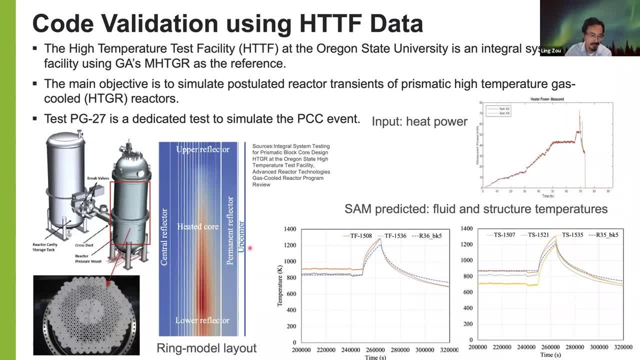 all this heat in the region and the permanent reflector and then all the way, All the way to the reactor vessel. What is not shown here is also, we have the RCC as panels here. So the basic idea is for code validation. 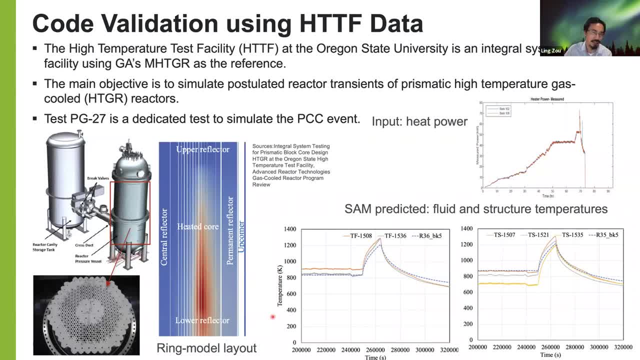 And there are a couple of the tests in the HTTF test, the suite we can use. So for this particular study we picked the test PG27, which is a dedicated test For the PCC event. So basic idea: here they have this heat up session. 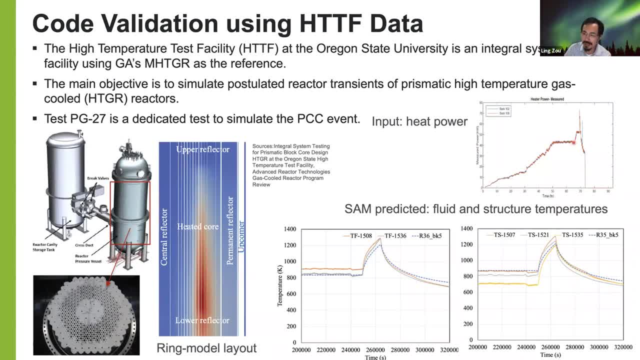 So they keep the heat up And then at some stage they shut down. Not really shut down, I mean to ramp down the heat to represent the decay heat behavior. And then I think here they probably just cut off the heat to simulate the decay heat curve. 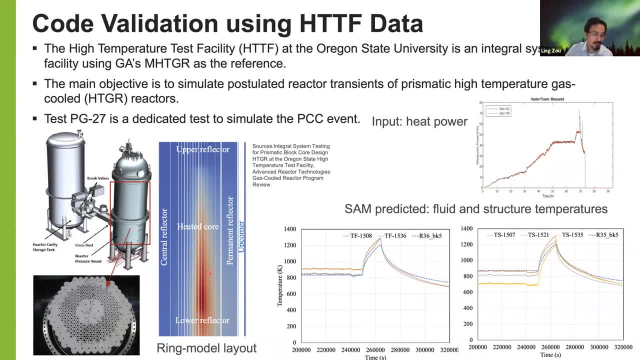 So basically we have- They have a lot of temperature measurement within the core and in the solid part. And here we model, I mean we predict. in this model we are able to predict both the fluid temperature and also the solid temperature. 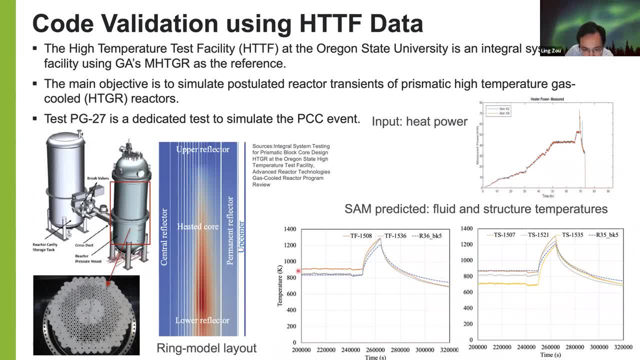 What here is shown here is: this is the pre-transient time period, And then you see It's like a pretty flat, And then this is the heat up corresponding to this part, And then this is heat ramp down and also this region. 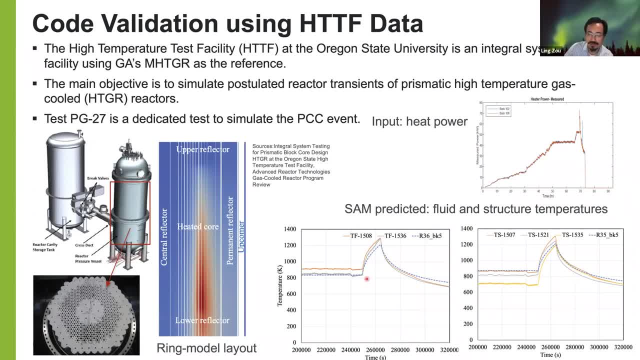 So what we can see here is that both the fluid and also the solid, the temperature is able to- I mean, agree with the test data pretty well. But of course we can see here is that if you look at the test data, 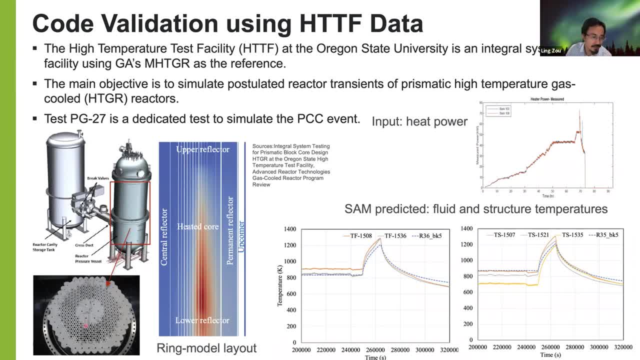 They're actually not. They should be. I mean, ideally they should be identical, because this core is like a symmetrical, But during the simulations, I mean during the experiment, it's not always the case, Because if you look at this flow channel, 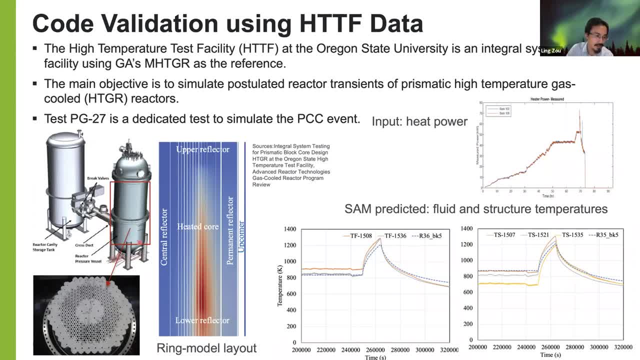 they're actually not with respect to this core. They're actually not perfectly symmetric. So that's why you see this kind of behavior. But in the 2D remodel, as we mentioned that we can we already assume that is perfectly exosymmetric. 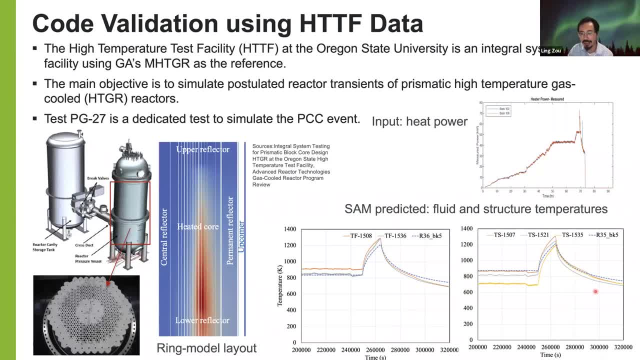 So we can only predict the one temperature. But even though you can see the temperature, both the fluid and the structure temperature, they agree with the experiment data pretty well. So we are pretty happy about what we are able to achieve here. So I think 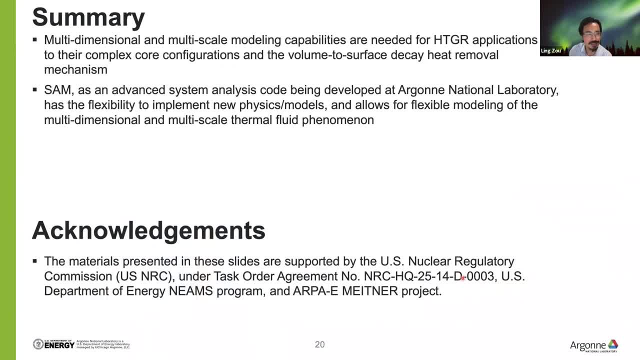 I think this is about today's presentation. I probably want to have a very short summary, So I think the key idea here is the HTGR, So they behave quite differently compared to the traditional reactor design such as the LWIS, PW and BWIS that uses a few rods. 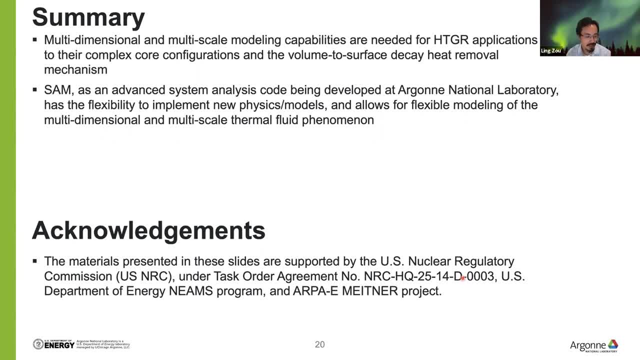 And then even during the transient, the heat transfer mechanism is pretty much the same. The difference is like a single phase versus two phase. But in the HTGR it requires this multidimensional, the multi-scale capability, Because when you switch from the normal operating condition, 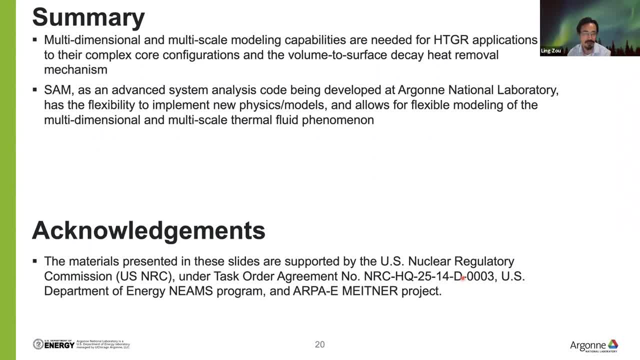 to the transient, then the dominant heat transfer mechanism. they change In order to capture such a multi-scale capability. there are some difficulties in the traditional codes, So at Argonne we are developing this new code, SAM, so as an advanced system codes. 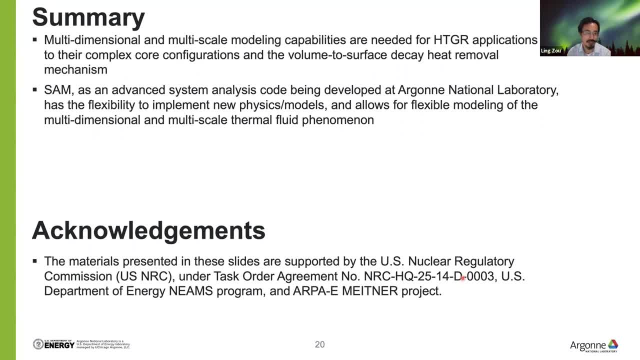 So we do have the flexibility to implement this new physics. As you can see in the explicit pebble bed, explicit pebble model, we have this new localizer, We have this new code and we are able to utilize the phenomena And we are able to implement them in the SAM user moose framework. 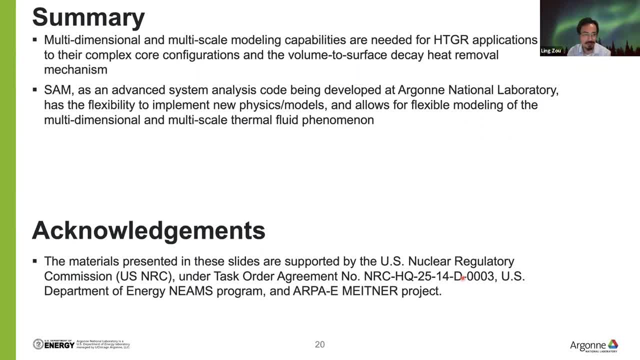 that allows us to do this kind of flexible code implementation. So with this I want to conclude today's presentation, And the final one is to acknowledge the funding support from the USNRC and also from the DOS NEMS program and some of the work shown in the slides. 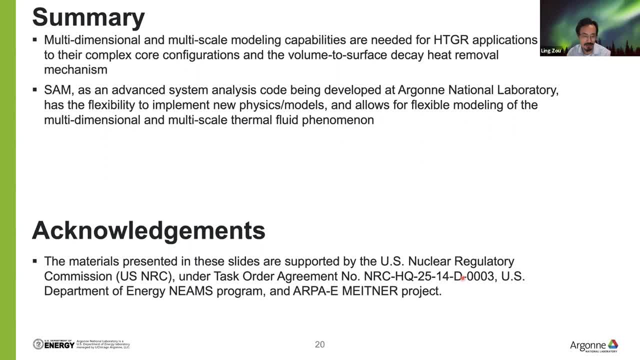 They are also supported by the APA-E mental project. With this, I would like to stop here And thank you for listening to this presentation, And if you have any questions, I'm happy to answer. So okay, thanks a lot for this very impressive presentation. 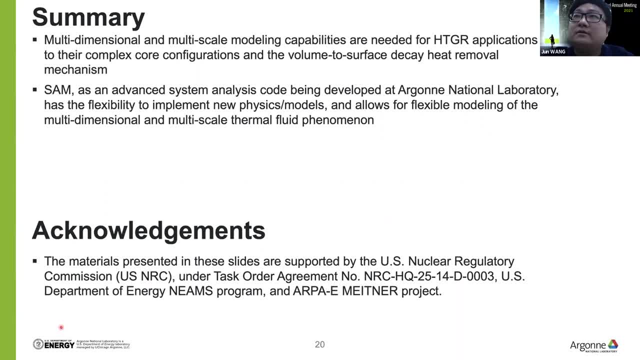 So do we have any questions from the audience? like Justin, Hi, that was a really great presentation. Let me just go to my notes really quick. Will you mute yourself? Oh yeah, I'm opening my notes. I know it's right now. 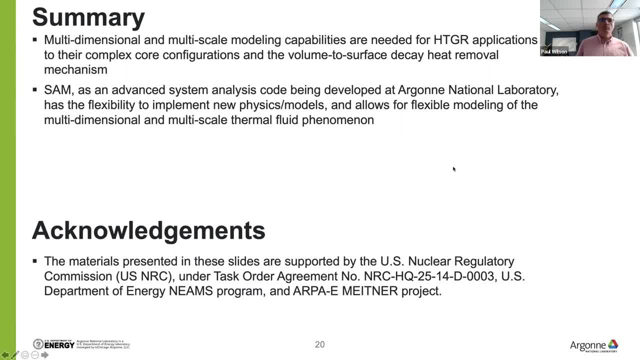 While he's doing that, maybe I'll have a quick question. So when you take a tool like SAM and some of the other tools, you've got a set of features And then you make some modeling approaches, as you described in various cases. 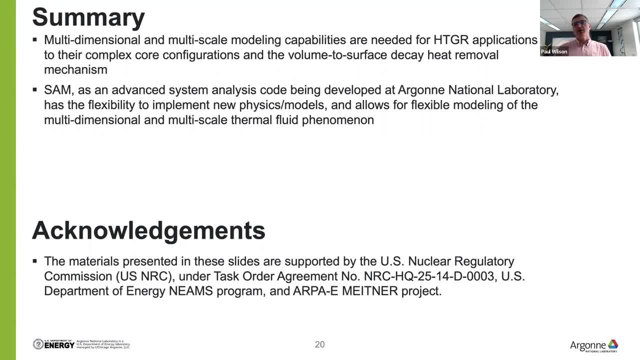 to model certain systems. At what point do those? if those modeling approaches are common across many different possible reactor systems or cases, at some point there's maybe an incentive for them to become a feature of the code. Do you understand the question? 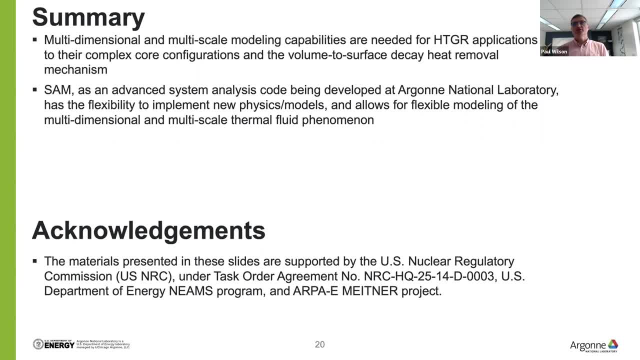 I will point to some of the sort of modeling choices and ways that you assemble existing features, get moved into the code and become a standard way of implementing a feature. Exactly, Yeah, I totally agree with you. Let's say, for example, the code, the SAM code. 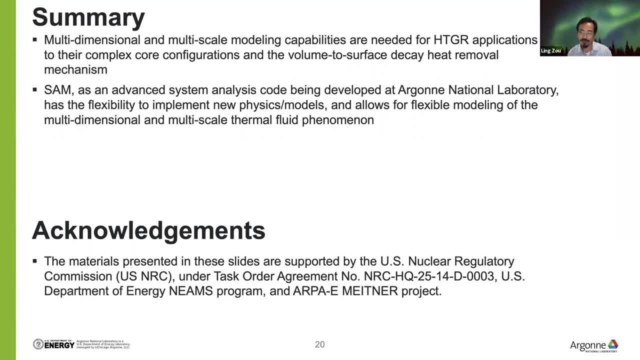 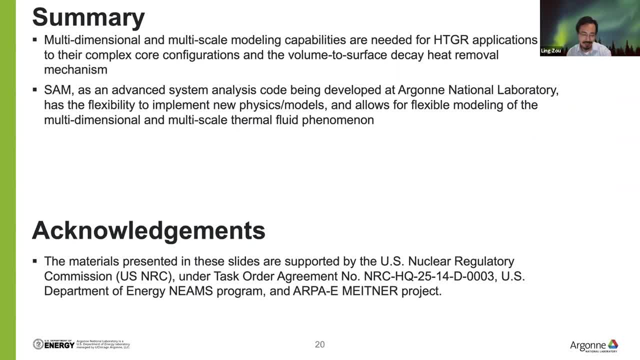 Of course, not showing the slides focused on HTGR. If we do have other kind of this, like you know, built-in capability to model, for example, sodium faster reactor. we have all levels of different components to support the SFAR design. 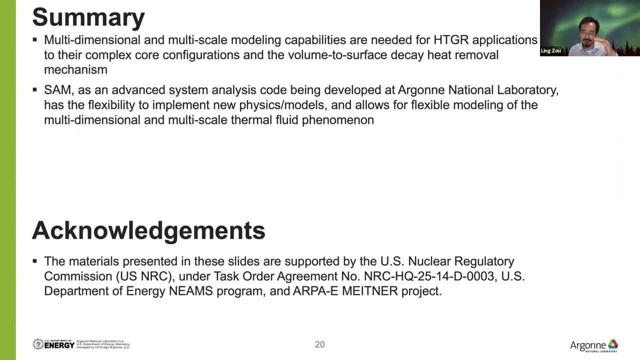 You have the very simple single rods. you know you can model for the SFAR single rod. Then we have this like built-in assembly. So, for example, you have a single rod, you can model for the SFAR single rod. 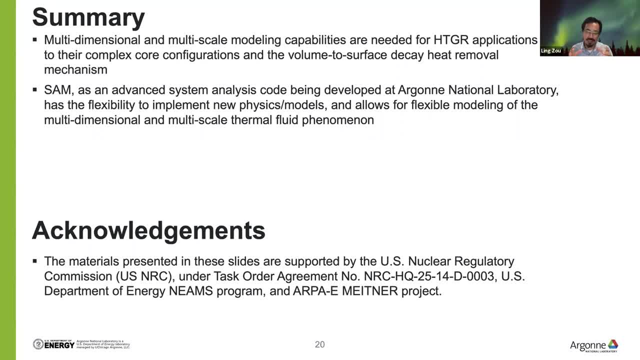 So, for example, you have a single rod, you can model for the SFAR single rod. So, for example, you have a single rod, you can model for the SFAR single rod. In the SFAR you have this like hexagonal fuel assembly. 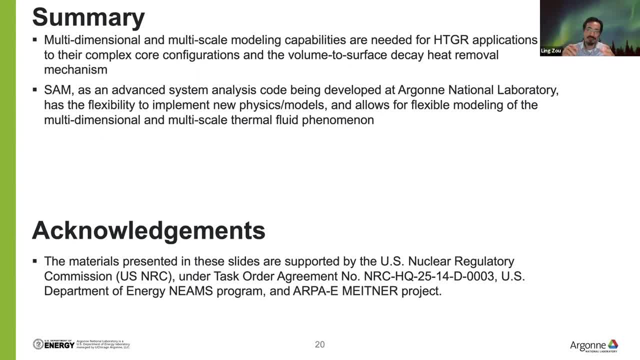 And then they are bonded in stainless steel box. You have this wire wrap handle, Of course. I mean as a user you can start in from one single rod and then build them one by one. But actually in SAM we do have such capability. 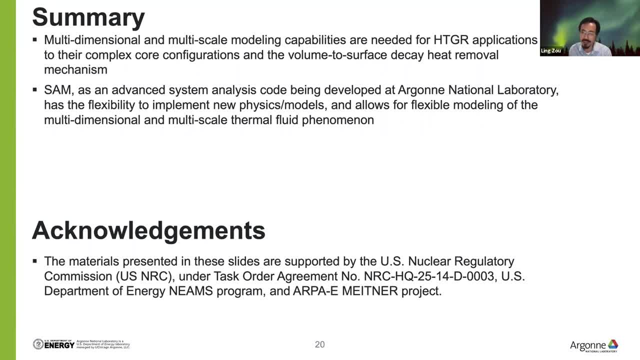 that to already to provide you this already built-in SFAR fuel assembly so you can just use them. And I agree with you that we can do the similar thing toward the, for example, HTGR, So, for example, if a lot of HTGR share the same similar feature. 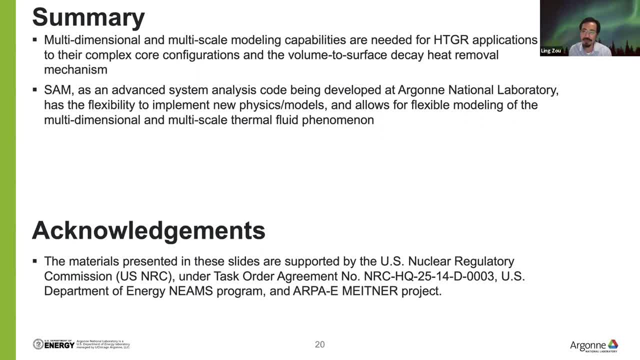 a common feature. we can definitely build such a pre-assembled component within SAM so the user can just use them to you know, like a Lego block. just put them together, Then you eventually do get it. This is something ongoing. For this one, we are still trying to explore the methodology. 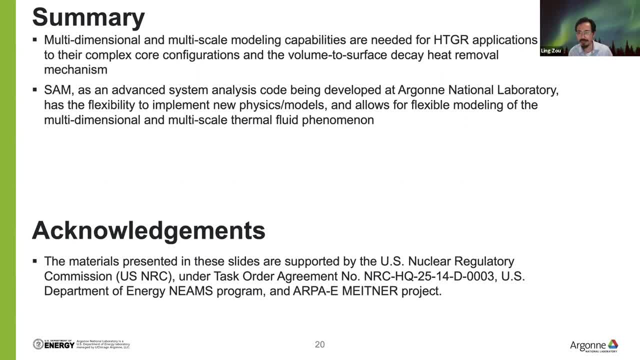 a little bit. You can see there's like a multi-phase of work here: One, we show the demonstration And then we show the two code validation. With this multiple phases, multiple stages of approach, we can start to build our confidence to say OK. 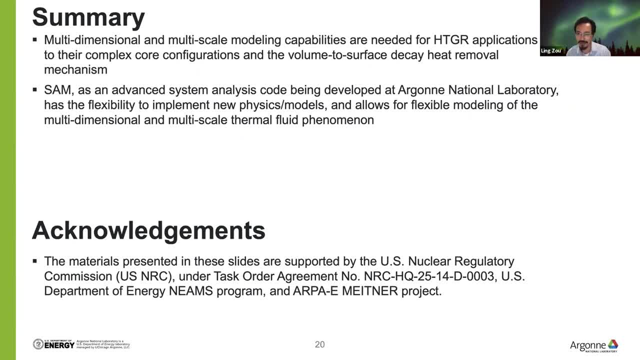 this should really be the way that you should model your HTGR system. Then we will go into this like code development phase to really to pre-assemble them, And that was a very good suggestion. Thank you, I was wondering. Oh, go ahead. 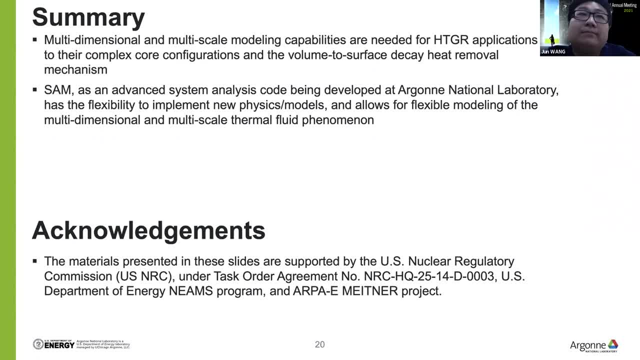 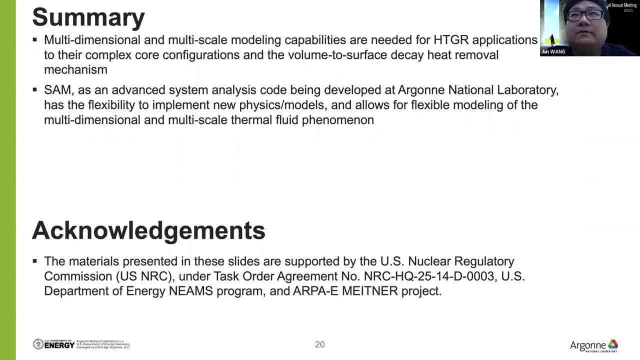 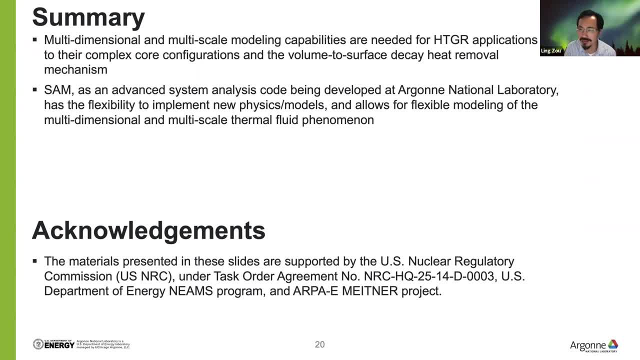 That's. that's also tied back to what Paul just mentioned- The user's menu, Rather than your modeling strategy. for example, here, the HTGR. we don't develop a new component, but we're trying to use this existing capability to. 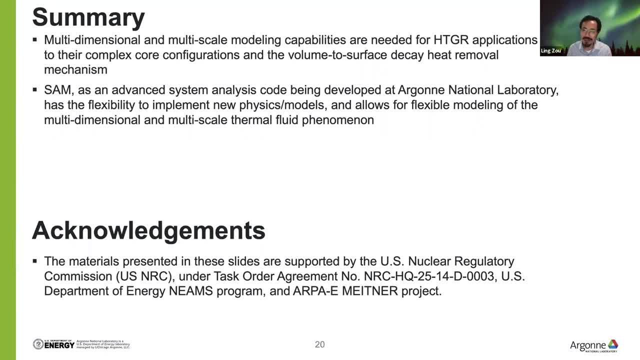 you know like a Lego block, you know like a user's menu. We will show you how does each of like block should work. but we are not. we normally in this user menu, we don't tell you how to build this model. 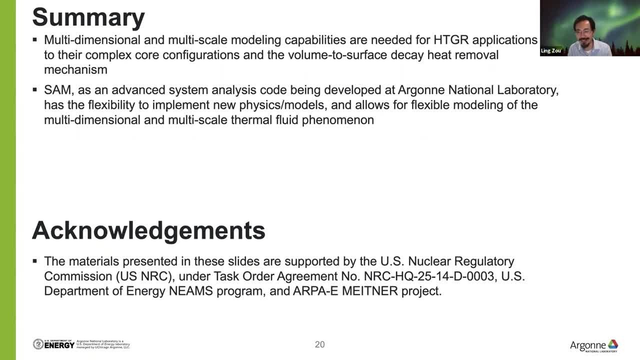 I. of course this is slightly different in the Lego story. cause Lego? they tell you how to build it. So we don't have a user's menu for how you build a HTGR model, but we have. we will have a report. 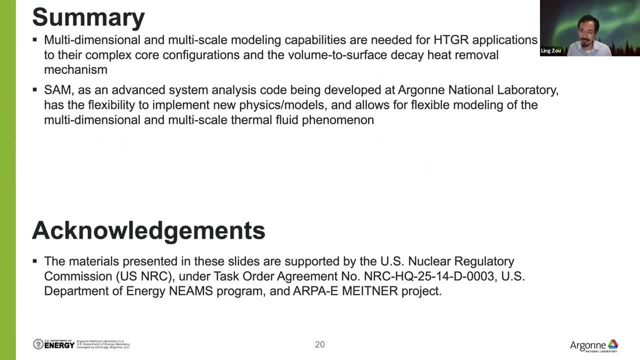 releasing very soon to explain what has been done behind the scene, how we decided to do so, why we believe this is the right way to do so. Yeah, yeah, You know. some user's menu include an example of sodium faster reactor and molten sodium reactor. 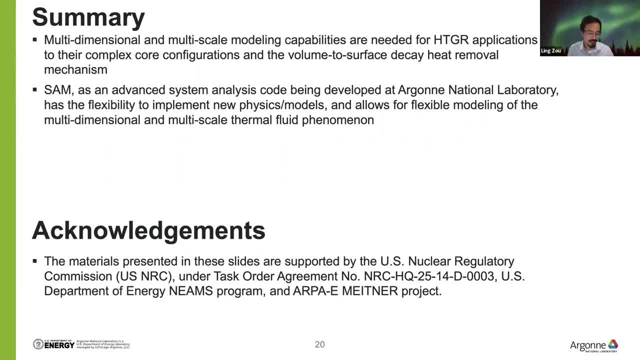 Maybe you can consider either one. Oh, okay, I see what you're saying. So you're talking about the very, at the very end there's like a demonstration section. Yeah, that's a good, that's a good suggestion. 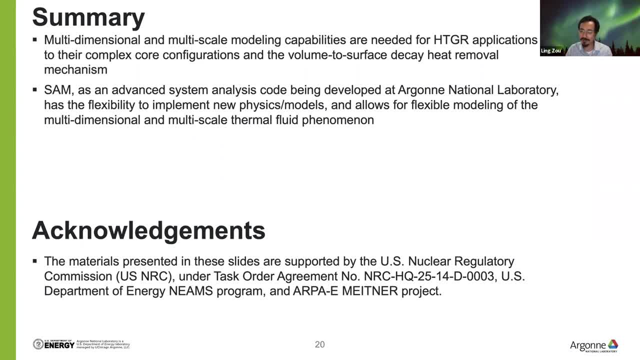 This is also, you know, the reason that Enric, the virtual test bed we're also trying to use, leverage that effort to, you know, to share the input files so everybody can use it, But of course without the menu. so, but you have reports. 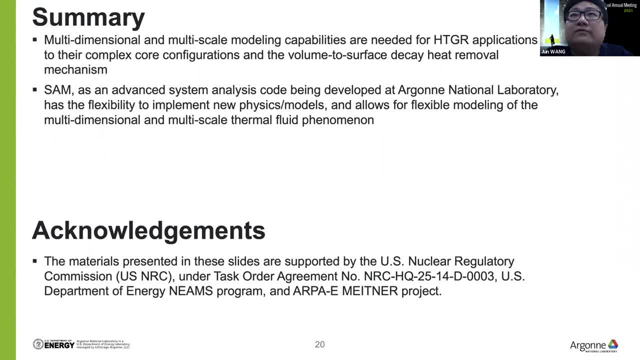 Yeah, and another thing is: I think you know there's a software called the SNAP from Enric. Yeah, it helps the users easier to use software like RealLife, Chase and Melco. So do you think it's possible in the future? 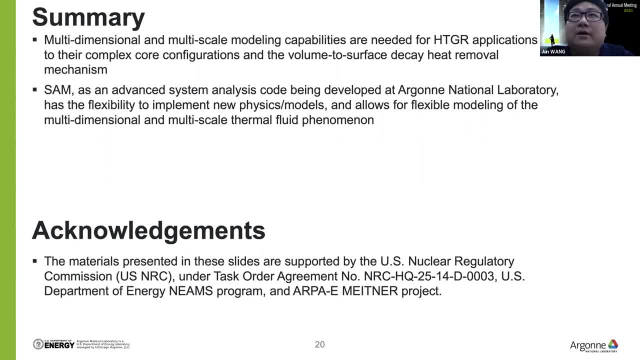 we can use SAM in the SNAP. So I mean it could be much easier for us to develop a new model. That's a good question, But the reason I mean for us, we're still focused a lot on the, you know. 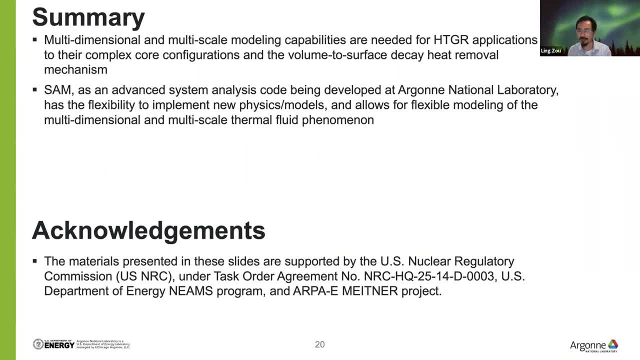 the capability, the code capability. Of course, what you ask is more on the UI, user interface side. So we- I mean the team, most of the team- really focus a lot on the physical side. So we are not there yet, to you know. 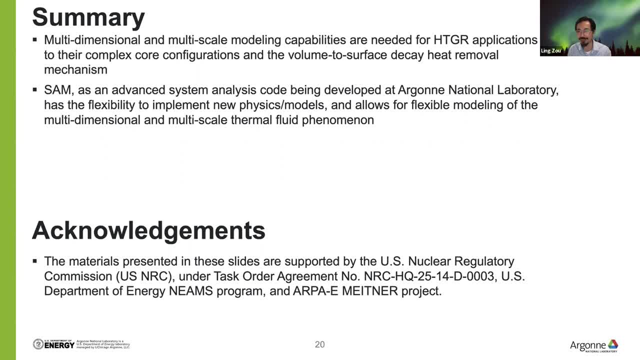 to have the luxury manpower to do this like user interface. Maybe in the future, when the time is right, when we say, okay, the code is very, very, very, very, very mature, now we really want to have the code have a good usability, then probably that's going to. 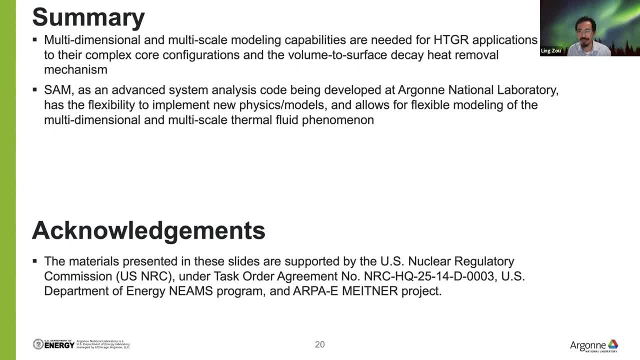 be the time to do this type of you know ui, but for now we do not have a like big plan to um to have this kind of um code, code implementation or code development. okay, okay, good, so, just yeah. so i was um. i found it really interesting about the 2d ring model design and how you can. 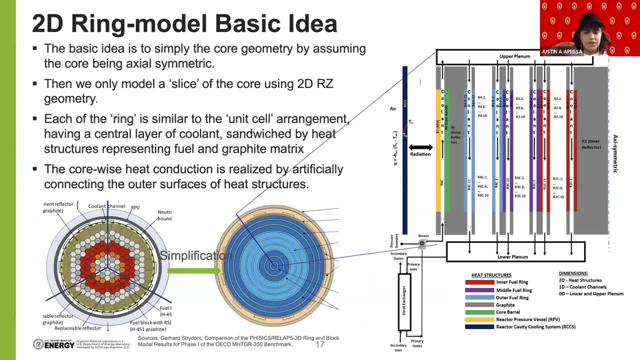 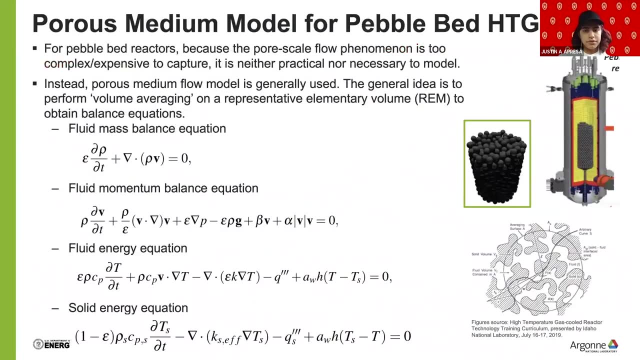 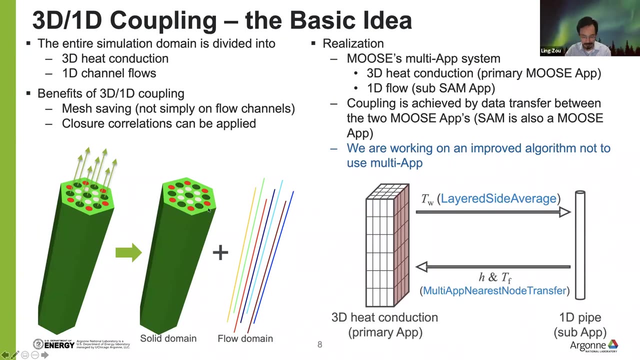 model. it helps make the simulation a lot easier. um, and then also, i was a bit confused about the um, the 1d and the 3d modeling as well. how do they mesh together? you were saying so. let me use this an example. so basically, this is the 3d, uh mesh. so basically, do i have a mesh here? so this: 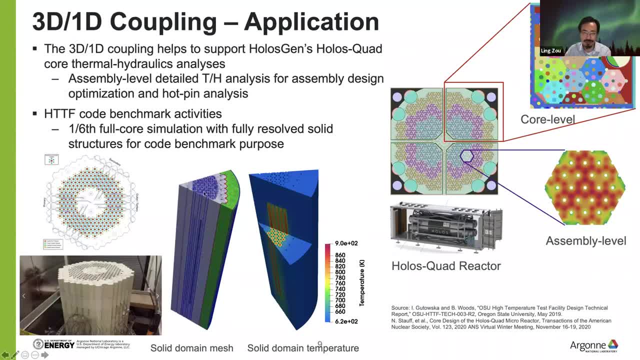 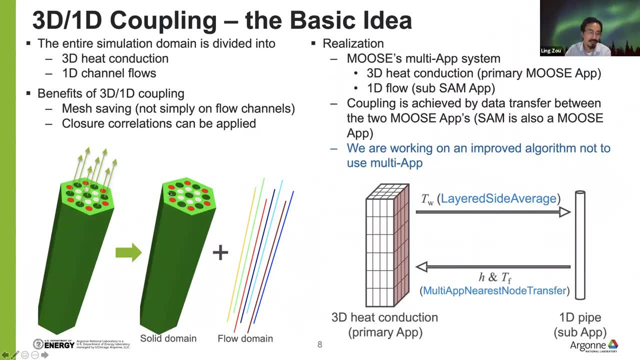 not the same thing, but you can see this is a 3d mesh. we do. you can imagine how i'm going to mesh this guy using similar thing. so we're not going to mesh. this thing is in the 3d heat conduction model. they're just uh, blank holes, but we know that there's like a coolant channel flow inside. 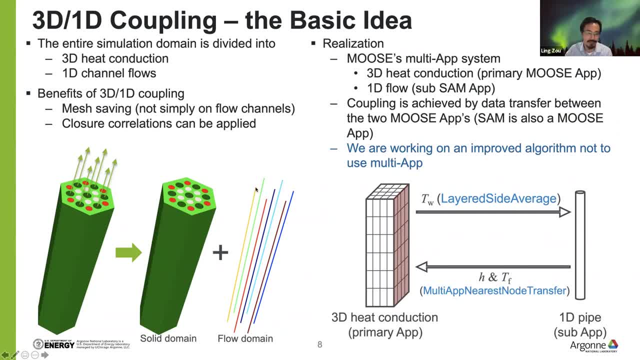 them and you want to model them. so in this case we use this, so, um, this like 1d flow model. so in each of this uh, you know this- holes, the drill, the holes, we have one of this like one dimensional uh flow. then let me move this thing a bit. so on this slide i did 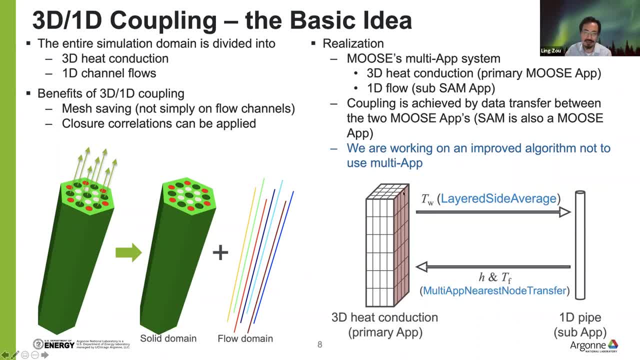 not, uh, spend too much time, but uh, really, what's happening here? you can see this uh red-ish surface. you can think of this as the internal surface of this hole, and then this 1d flow channel is like a this flow channel that's talking to this hole. so basically, the idea is that 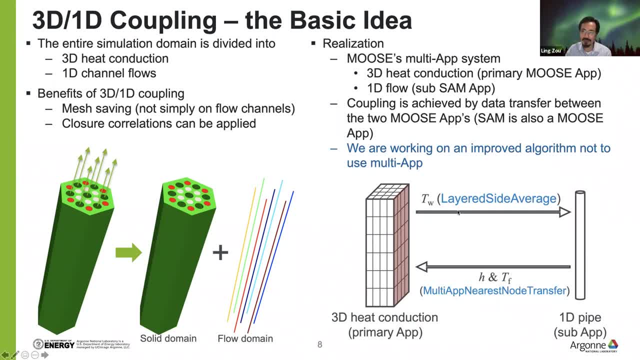 this run. actually they are running in two moose applications, if you are familiar with moose. so basically you can run two input fires and then they talk to each other. we do not, uh, we do not tell. i mean, we just tell them how to talk to each other, but we do not. 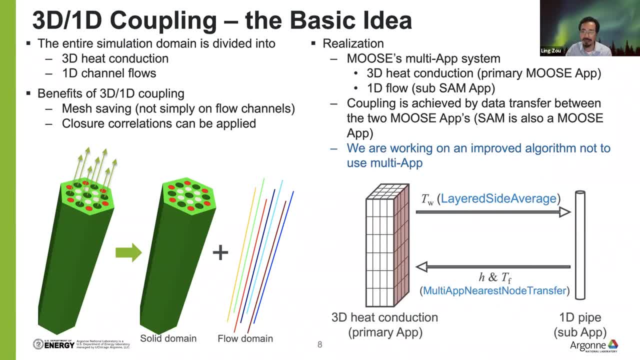 do any encoding, implementation or anything to implement anything, to let them talk, because moose makes them talk. so, um, with this kind of infrastructure, we can let them talk to each other. so we will. um, in this case, we will have this t wall, which is the average surface temperature of. 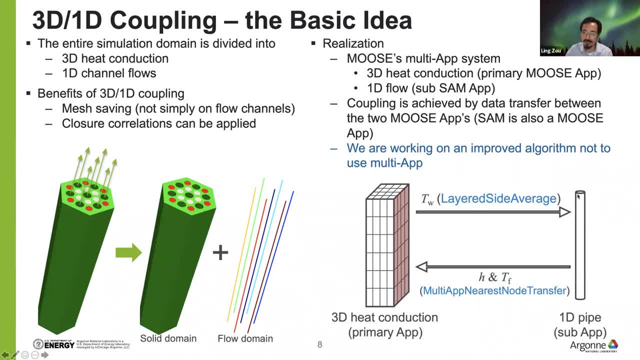 this red-ish surface and then transfer this temperature into this coolant channel. so the coolant channel knows that it is talking to this red-ish wall and then, either way you use this wall temperature to compute, you know like the heat transfer, you know like a use, sometimes it also used for the uh correlations and then when the com does some compute it, then 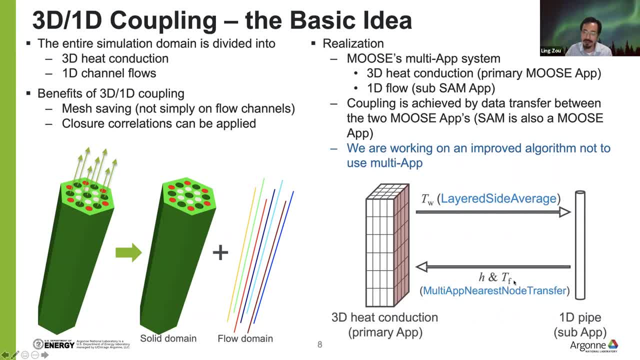 knows the, the heat transfer coefficient, and then it will also transfer back the fluid temperature back to this surface. so you can see this like information exchange, and then that requires some internal um, picard iteration and um. so for this particular algorithm we are not taking advantage of this newton's method, but we are working on an improved algorithm. 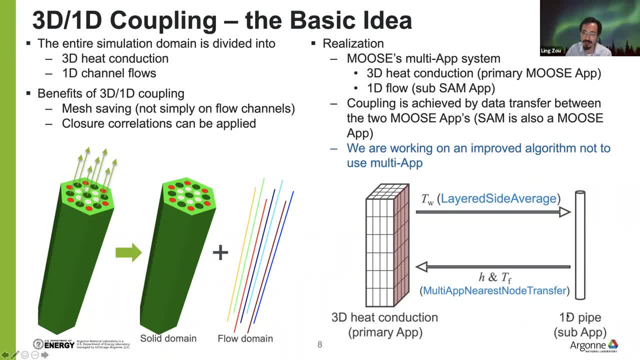 not to use this multi-app, but we are going to put them all together in the big newton's um uh iteration so they do talk to each other, but they- we do not need this like internal uh picard iteration, so that will save us. save us a lot of like computational time, because you understand. 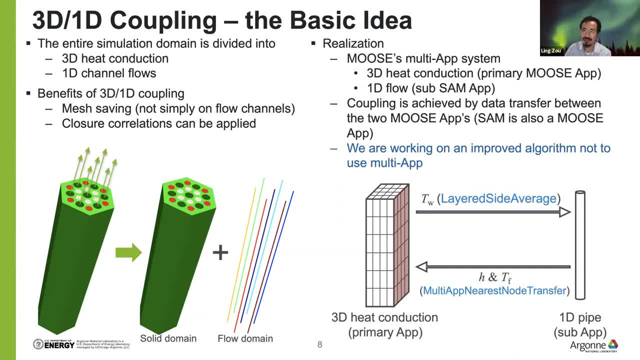 picard, iteration sometimes can be nasty and the time can swim. okay, that's what i was wondering: just how they would talk to each other, because i i understood that they were separated, but i didn't know how they would talk to each other. okay, they are behind the thing. basically, moose controls that. so we just say okay, so you just tell moose. 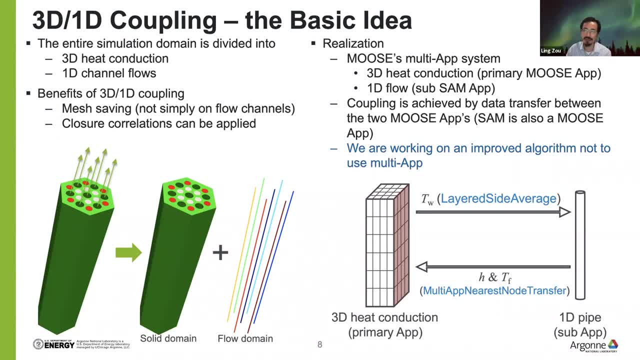 what kind of information you want to transfer. moose would do that for you. okay, in this case. in this case, we believe moose does a good job because i mean you know, when we do code, the validation, we we know they are doing a good job. otherwise, when you do kind of validation, it will not be to show good results, okay. 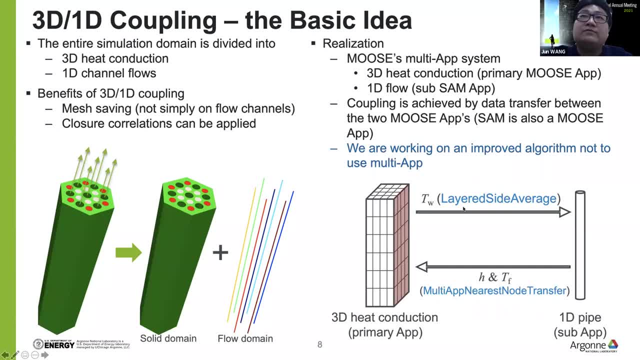 okay, so if we don't have other questions from the audience, please thanks again for dr zou his very great presentation. thank you very much and hope everybody have a great afternoon, thank you. thank you, jim.